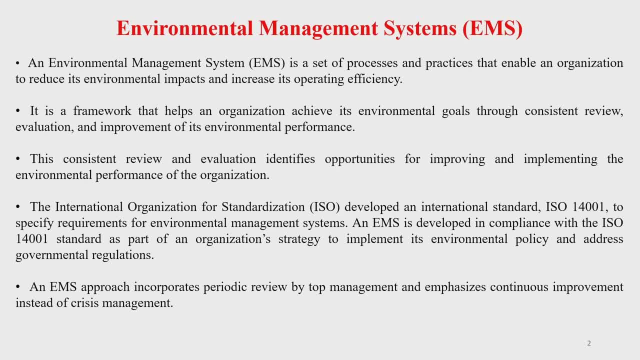 its environmental goals, like green environment, good water, good soil, suitable amount of biodiversity- These are the different environmental goals- Through a consistent review, evaluation and improvement of its environmental performance. When we say environmental performance, it means that the resources that we will be utilizing. 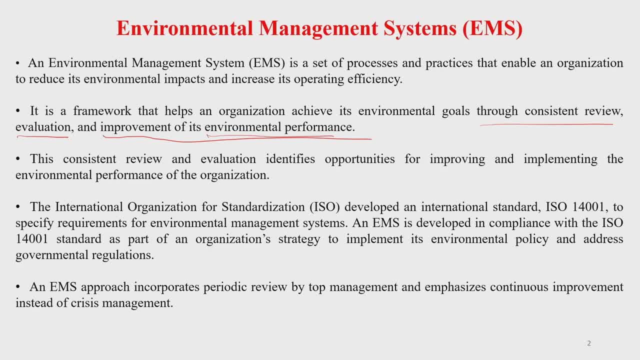 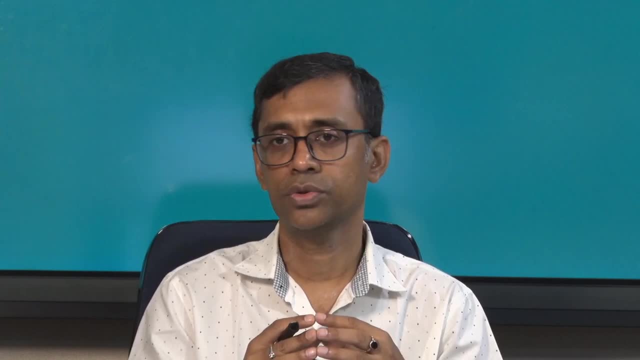 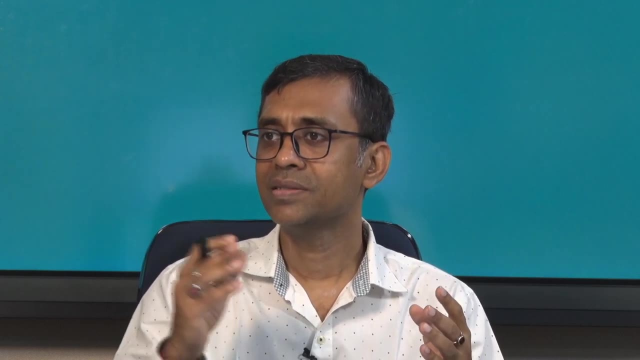 for our sustainable living in any community or any locality, We need to see that utilization of these natural resources is optimum, and we are also taking care of its regeneration wherever it is possible. So the utilization of natural resources will be in sync with the environmental management. 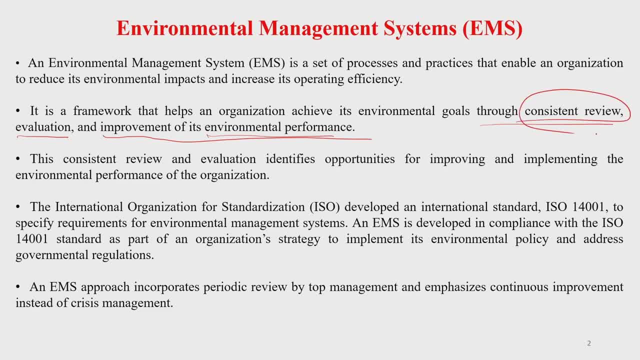 Now, when we say about this consistent review, this consistent review and evaluation identifies the opportunities for improving and also implementing the environmental performance of that community or organization or group. Now there is a international organization for standardization which we call as ISO. Many of you might be knowing about this. ISO developed an international standard which 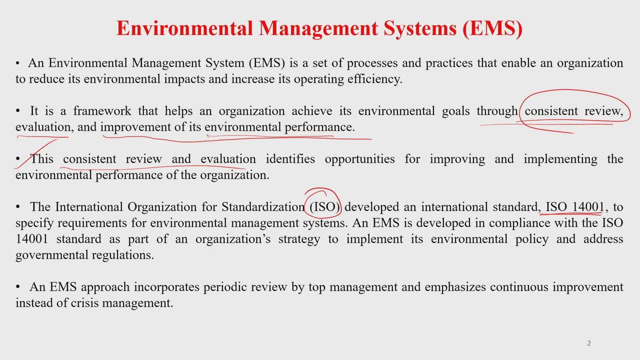 is followed by certain numbers, like ISO 14001 here, which is does is specifies the requirements for environmental management system. It tells us that how and what should be the approach, and it also gives us certain numbers and values which should be followed if we are trying. 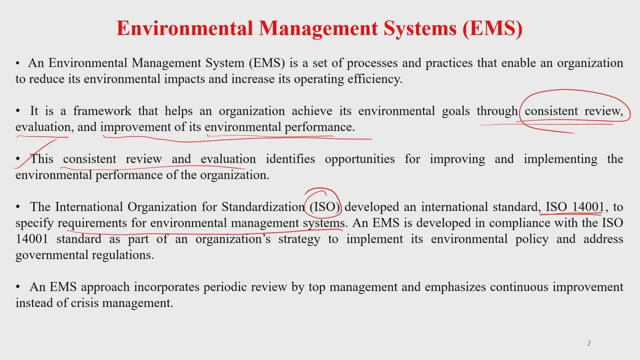 to do appropriate implementation of that particular ISO system. under environment management, An EMS is developed in compliance with the ISO 14001 standard as a part of the organizational strategy for what to implement this environmental policy and to address the government regulation. Like many other countries, in India also we have various environmental regulations rule. 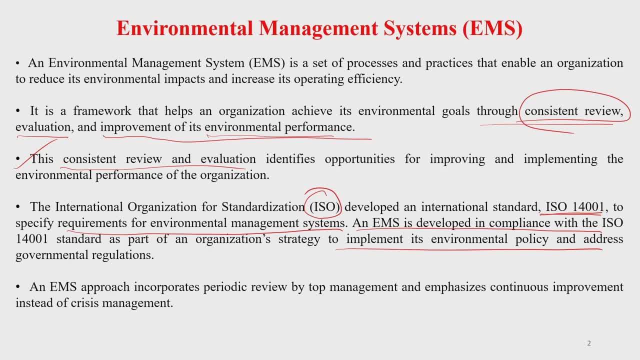 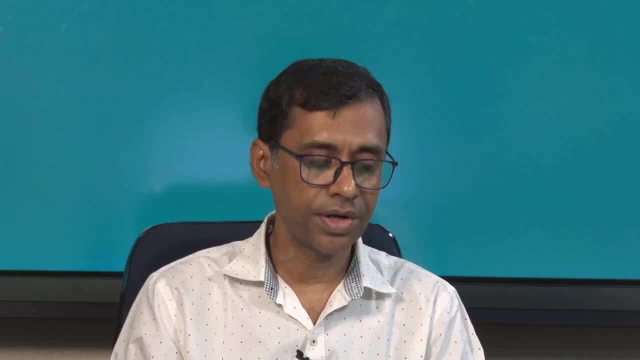 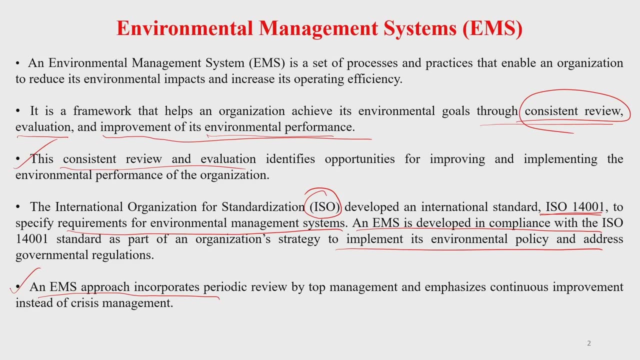 and also we have a tribunal, national green tribunal. I am sure most of you have heard about that. We call it in brief NGT: very powerful authority to protect our environment. An EMS approach also incorporates the periodic review by top management and emphasizes the 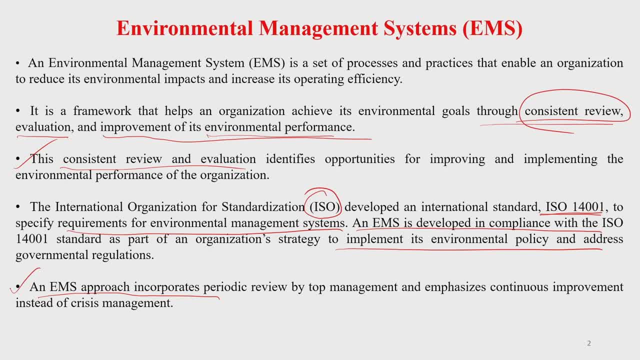 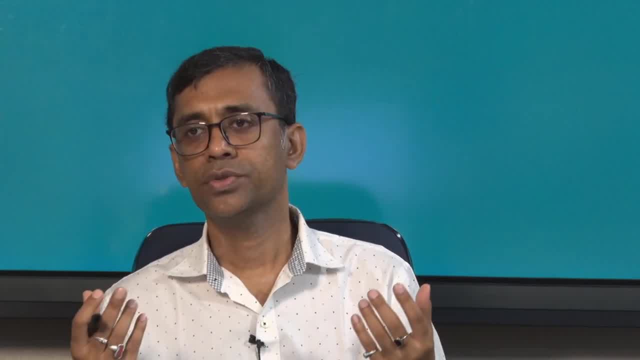 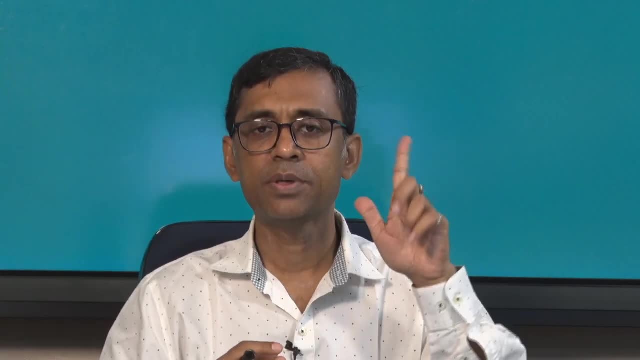 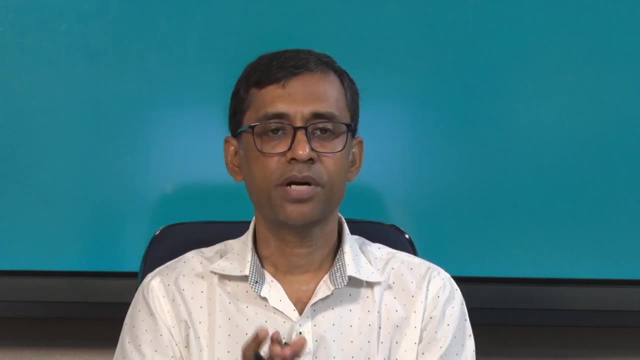 continuous improvement instead of emergency management or crisis management Means because of, suppose, our continuous utilization or extraction of a certain natural resources from the ecosystem. if there is a negative impact on the environment suddenly happens and we go that and manage that kind of a emergency purpose. that is not the objective of EMS. What we need to do is that we need 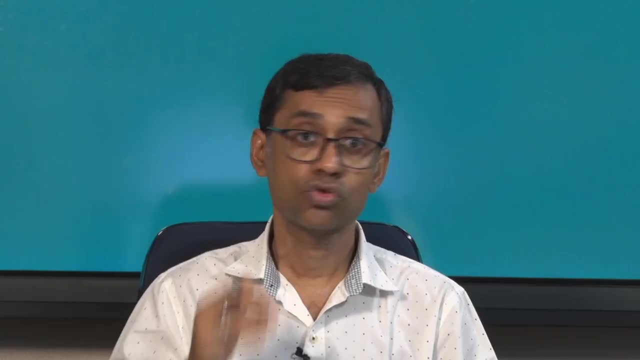 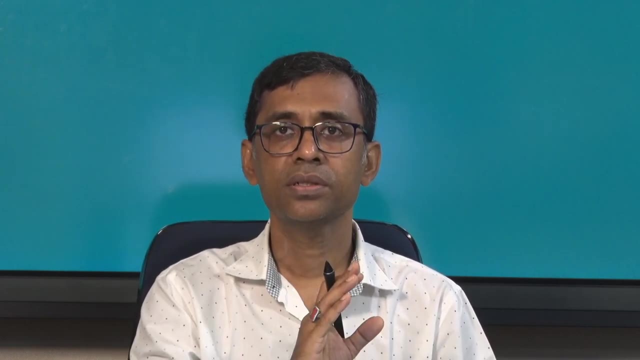 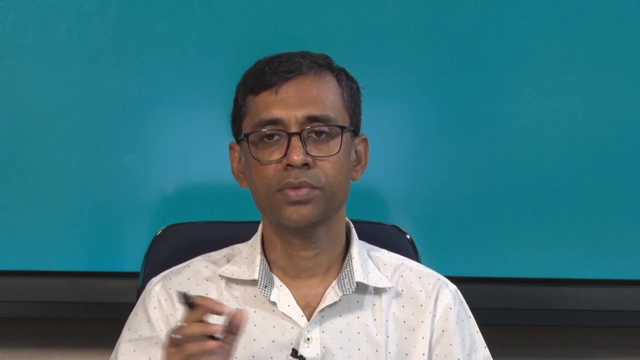 to have a consistent review of the process so that that kind of emergency situation should not even arrive. So, in a sense, prevention should not even arrive. So, in a sense, prevention is better than cure. So we need to be prepared through consistent review, evaluation of the 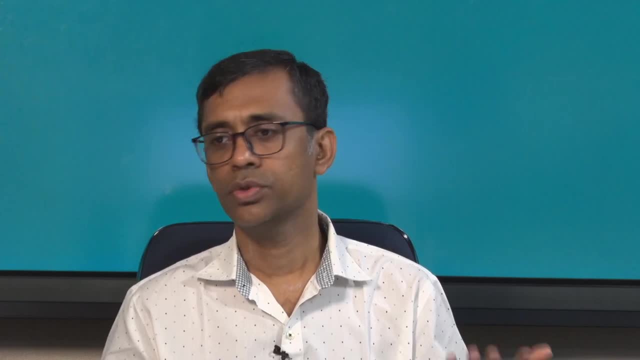 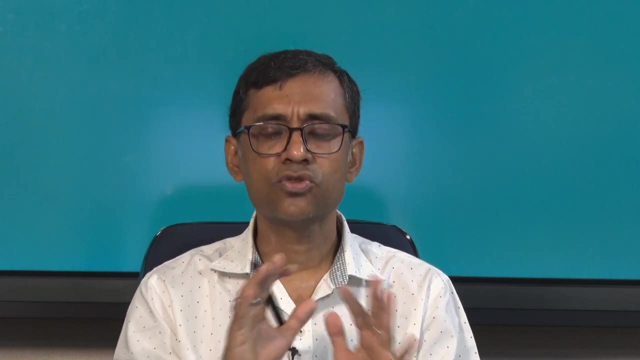 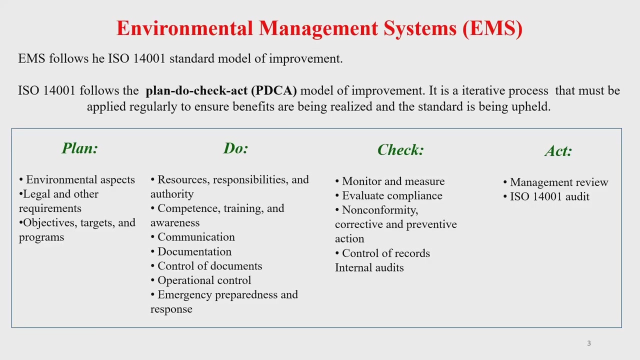 system because we know that natural resources we will be needing, we will be continuously using it. but how, when and how much, that needs to be actually reviewed and accordingly the system should be managed. Now EMS, as I said, that it follows certain, certain ISO. 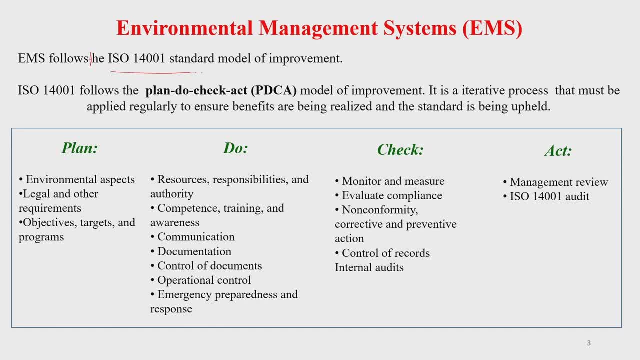 standard like ISO 14001 is a very standard model of environment. you know improvement ISO 14001 follows the planned, do check act. We call it PDCA model. plan: you plan, your action, you do or carry out, you cross check that how it is working if there is any fault. 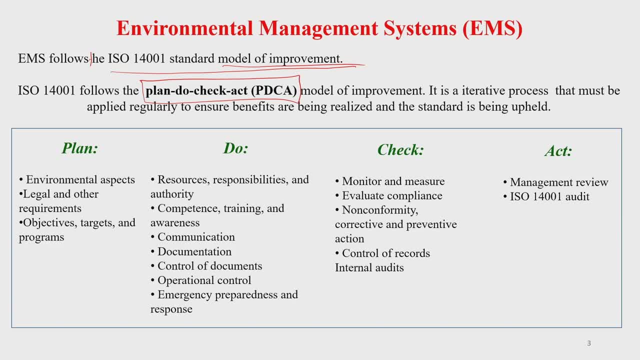 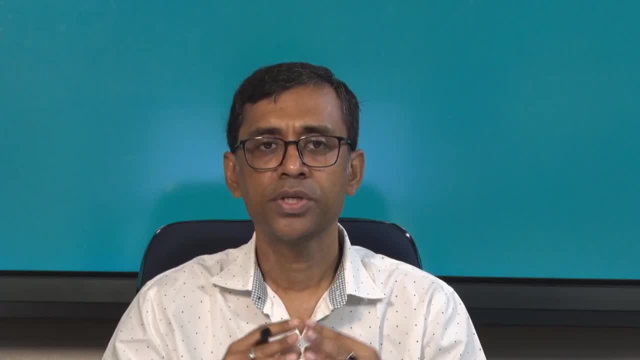 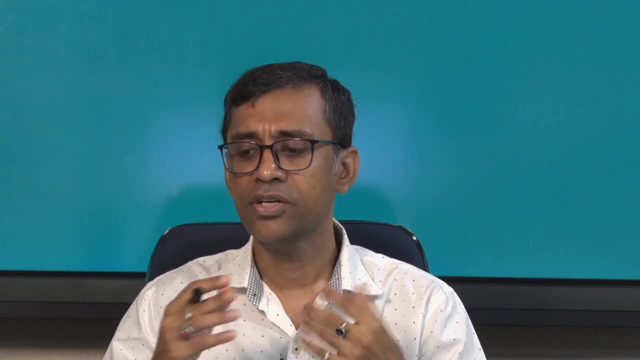 act implement. So this PDCA model of improvement under ISO 14001 follows the plan do check plan in 1001- is very, very important for appropriate environment management and so natural resource management. It is a kind of a iterative or repeating process which must be applied regularly. 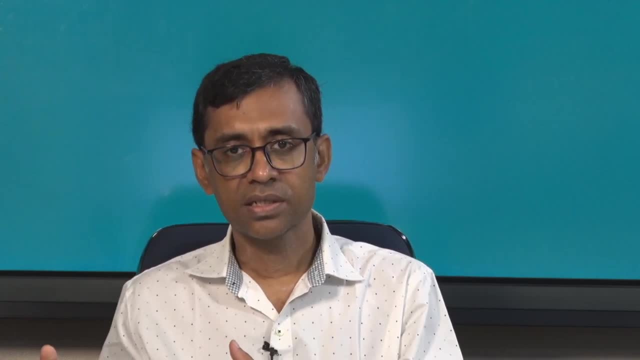 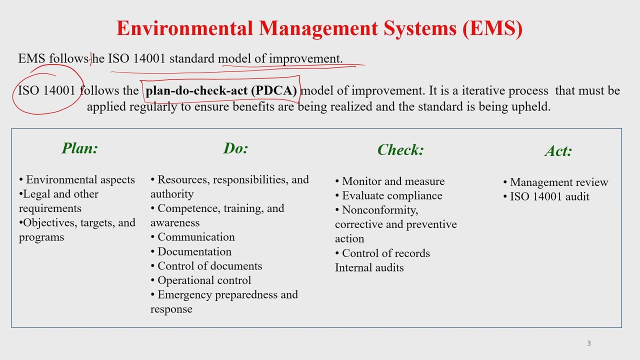 to ensure the benefits are being realized and also, at the same time, the standard is maintained. Now let us see how these PDCA model you know work. what are the various aspects of this plan? do check and act model plan. first step, What you do here. you actually look at the various environmental aspect associated with. 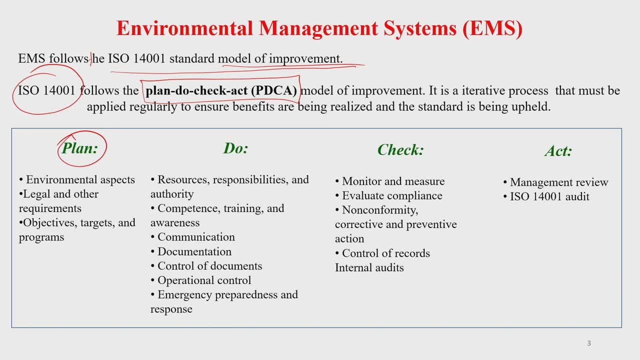 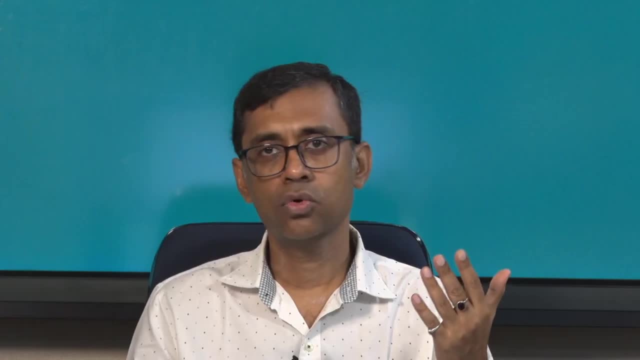 any act or any activity that you are carrying out in a particular locality, You also look at the various legal- you know- angles associated with that. say, for example, coal, Coal, Coal, Coal, Coal is a very important natural resource and suppose in your locality there is a coal. 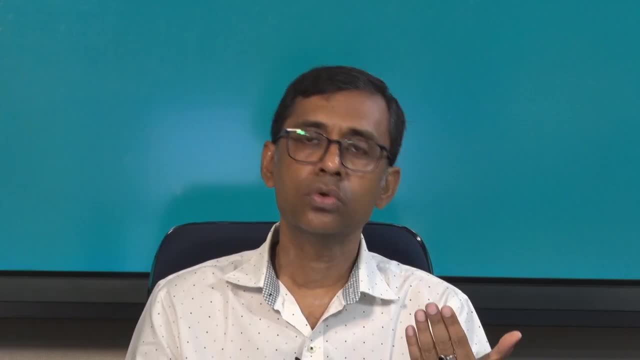 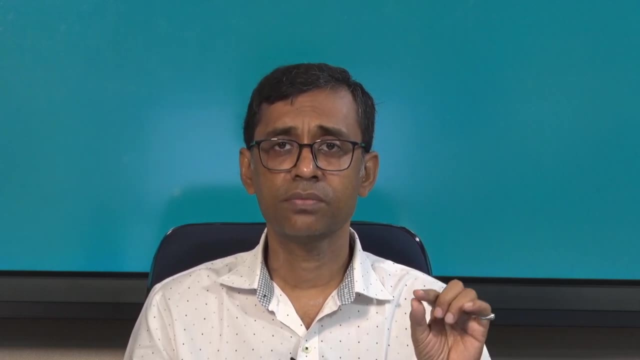 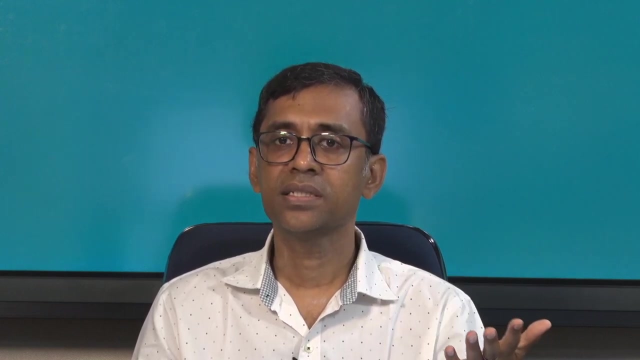 mine and coal mining is going on. We all know that coal mining should not be continue beyond a certain limit. There are several aspects of environment. concerns are there and then, of course, the- you know- safety issues related with land and various other aspects. So we 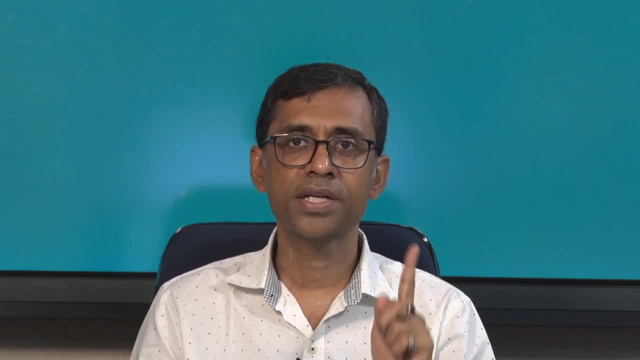 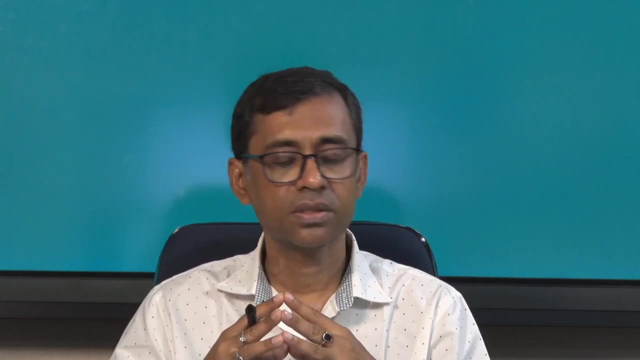 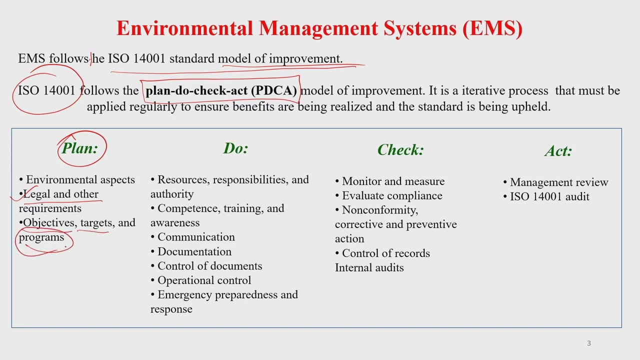 must see follow the rules. So the mining process is associated with also the mining process. You know I have just taken an example of mining, but it can be applied for various other aspects of natural resource management. Then comes your objectives, your targets and programs. Say for the example: 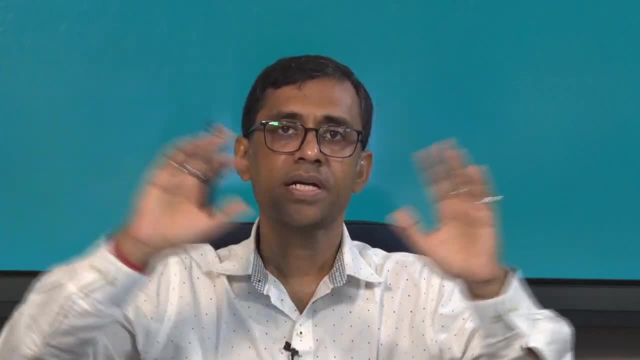 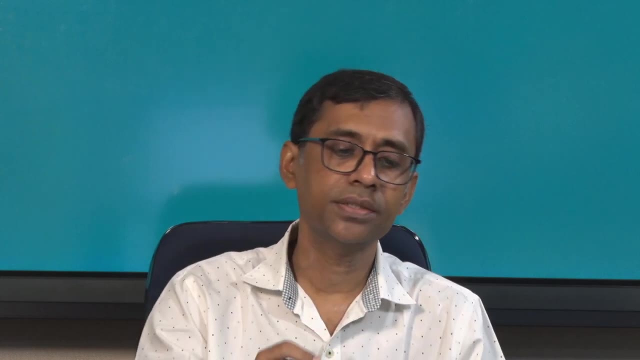 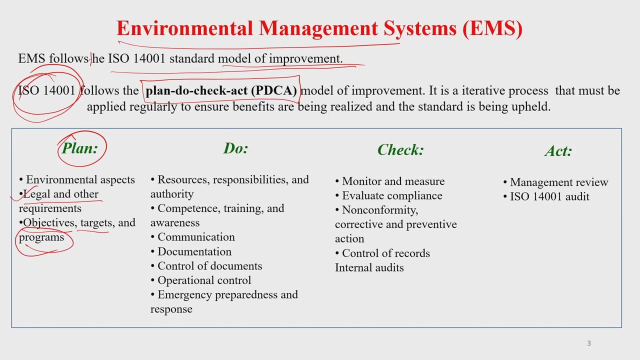 of mines I have given. So you have a target right. any mining company will have a target that how much are need to be extracted you know from the ground. but these all should be planned in accordance with certain rules and standard to keep our environment safe so that the human life and the ecosystem does. 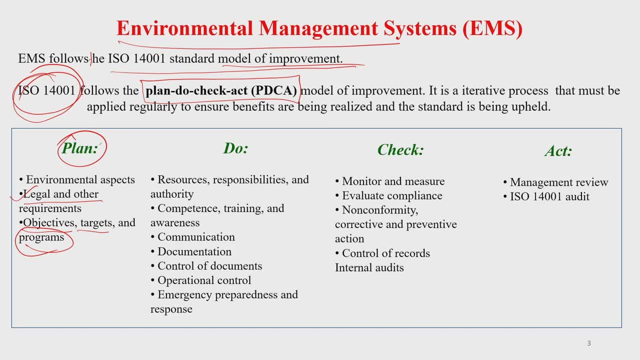 not come under any kind of danger. Once plan is done, then you go for doing it. What are the things and how you do that? See all the resources that you have at your disposal. you should utilize them responsibly. I mentioned it at the very beginning of this course that responsible utilization of natural resources. 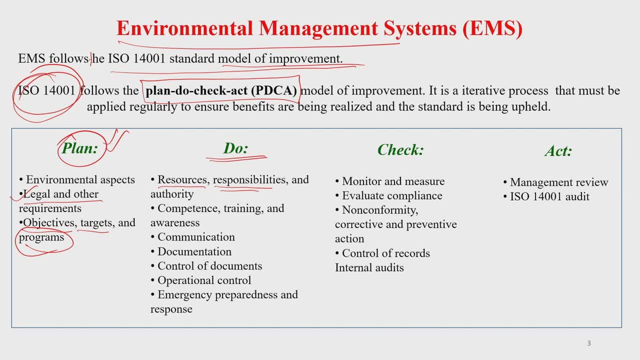 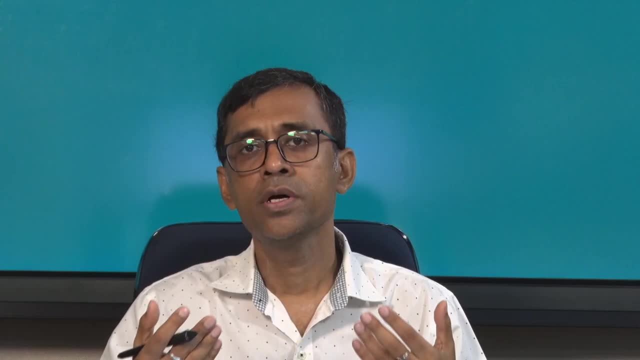 is one of the key aspect of an efficient natural resource management regime. Now authority: when, say, some government department, some organizations who suppose own mining area or a mine, they also will have certain amount of responsibility, because any authority that comes with certain responsibility. 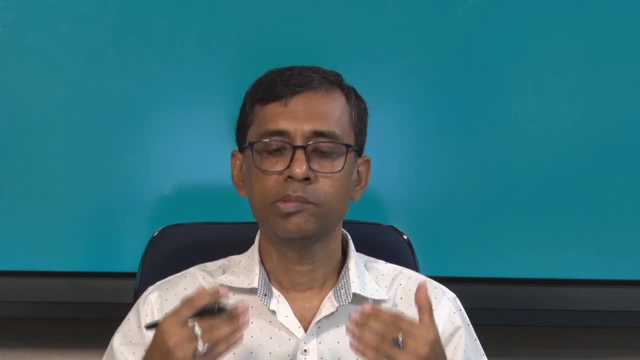 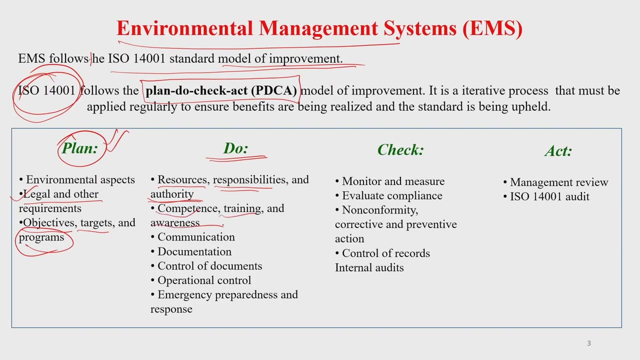 So it is their duty to see to implement the certain aspects associated with environment management system. Competence training- awareness, of course, is very important- and these all those things you will be actually doing during your actual ground work. Communication documentation. 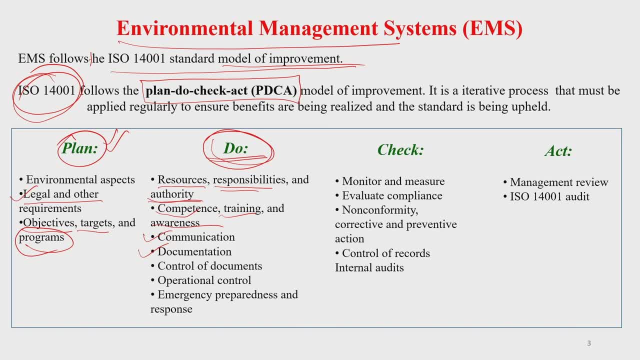 you know, periodical review report and different kind of leaflet, control of documents, operational control And emergency preparedness and response. So these are some of the you know points activities that will come in the second step, that is, do out of PDCA model. Then comes the next. 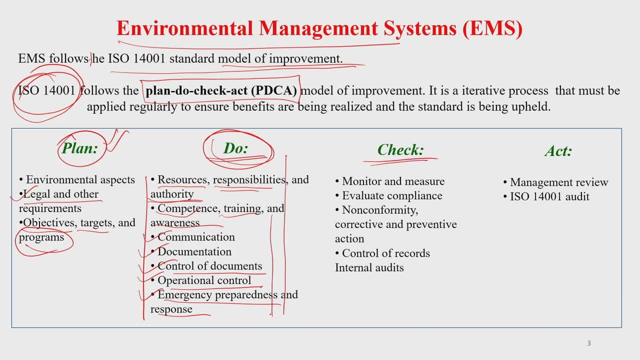 step check. So once you carry out this set of activities, then you go and check your system how it is work, and that you do through a continuous monitoring, evaluation measurement. Then you try to find out any kind of non-conformity, corrective actions, preventive measures that you take and control of records. 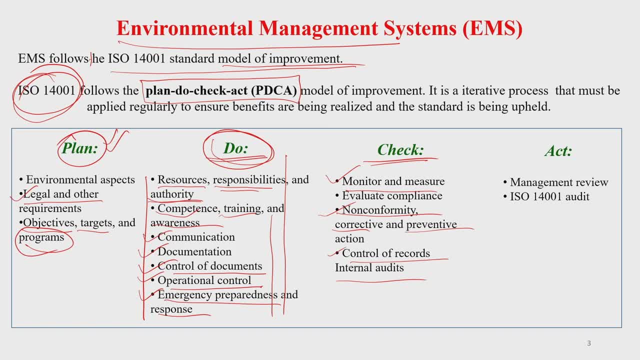 internal audits. These are some of the important aspects which comes under check. you know, step of PDCA model And then finally comes act means this is the step of action. So there you actually, you know, carry out a management review of the entire system and activity. and you see, 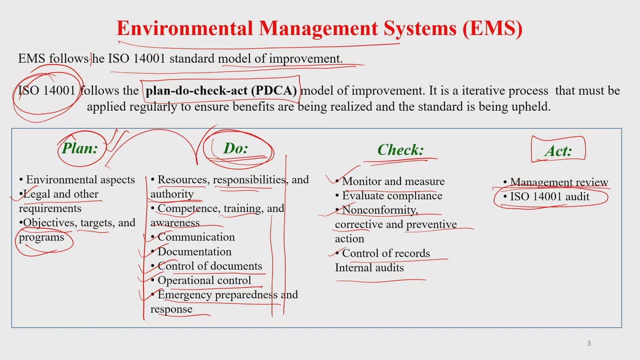 that how much your all this planning, doing and checking exercises have, finally, you know, help you to implement the ISO 14001, you know- system, or any ISO standard system as approved by any government of a particular area, has been implemented appropriately. 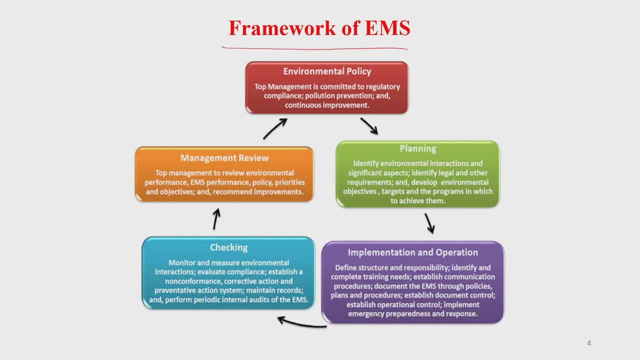 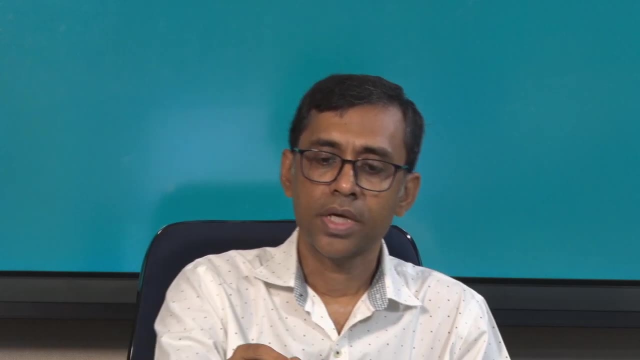 Now let us look at the framework of EMS, environmental management system, Environment: any environment management system or EMS, it has certain component. On the basis of those components, EMS work in any ecosystem. What are those? Environment policies? any location or place or country. 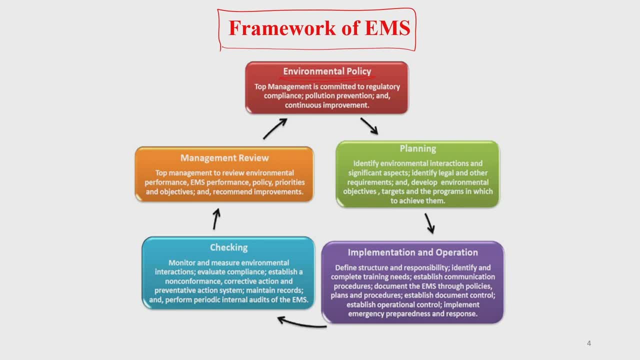 or state will have certain policies associated with environment and when any company, organization or group comes to work in any locality, the top management or authority of that particular group or organization supposed to be responsible committed to the regulatory compliance of the set of rules. 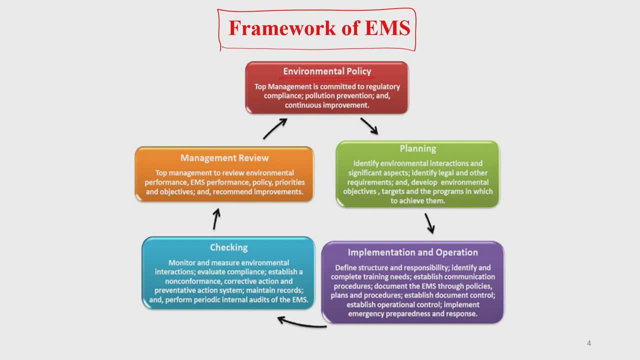 for proper environment management And that those actually, you know, include all kind of pollution prevention, different kind of measurements to reduce the pollution, continuous improvement, evaluation of the system, as I just discussed in the previous slide. So once you have this kind of policy, on the basis of that, within EMS framework, one has 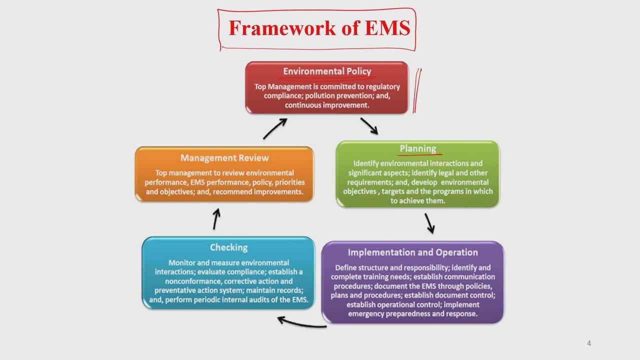 to do a planning where you actually will identify the environmental interactions, then identify the legality, legal aspects and other requirements associated with that. Then you develop environmental, you know objectives, which are the thing that you would like to do in a particular area, because, location to location, the type of natural resource, 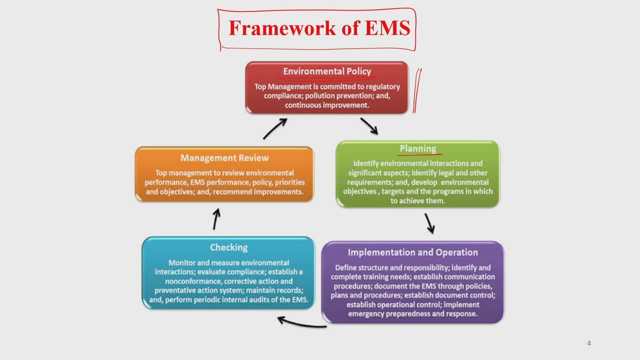 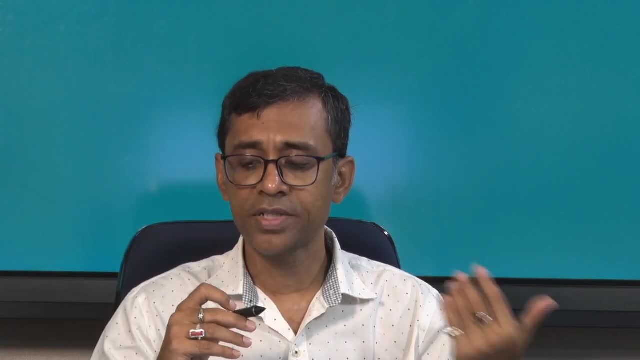 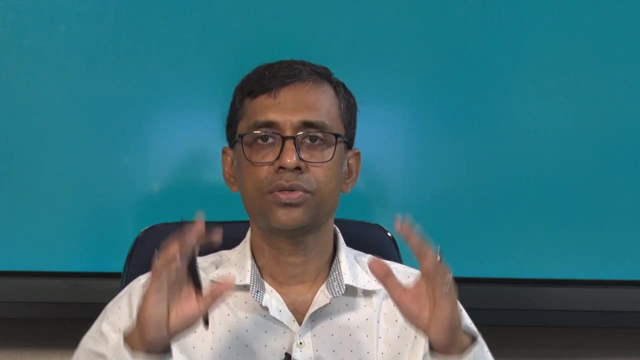 utilizations will be different, So on that basis, certain strategies will also differ from place A to place B. So then you have targets and the programs in you know, through which you actually try to achieve the goal. The goal is to have a, you know, sustainable. 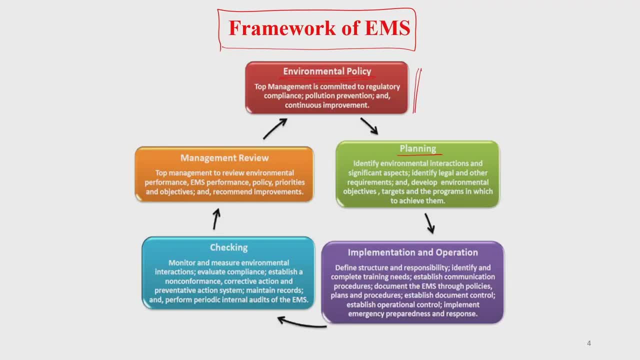 environment management system in place. After planning, then you go for implementation and operation. In case of implementation operation, as we discussed in the previous slide, you actually define, you know, structure and responsibility of each individuals and each individual organizations responsible for that particular task. You. 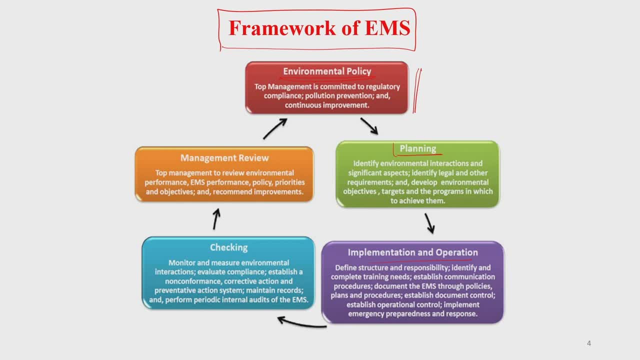 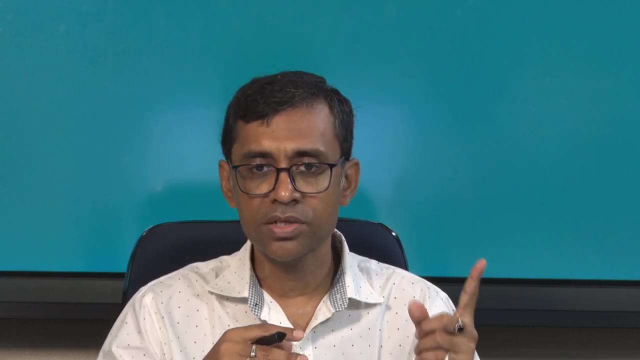 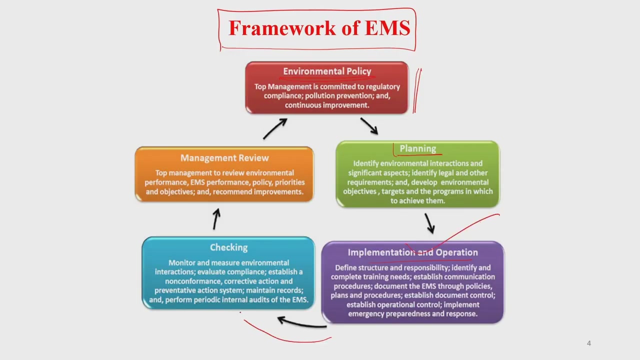 establish a communication network, procedures, how to communicate between each layer of responsible people and authority, document them, carry out, you know, awareness program, establish different kind of operational control And then implement emergency preparedness. you know plan of actions and response. Once this is done, then you go for checking, as we discussed in the previous slide, where 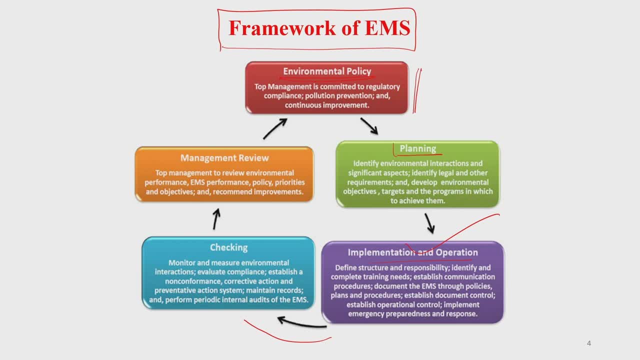 you carry out largely the monitoring and evaluation aspect to check that how much actually it is following the standard that has been set at the first level Once the checking is done, and then you find that if there is any kind of gaps or any kind of corrections that could be carried out, you have to carry out that before you reach. 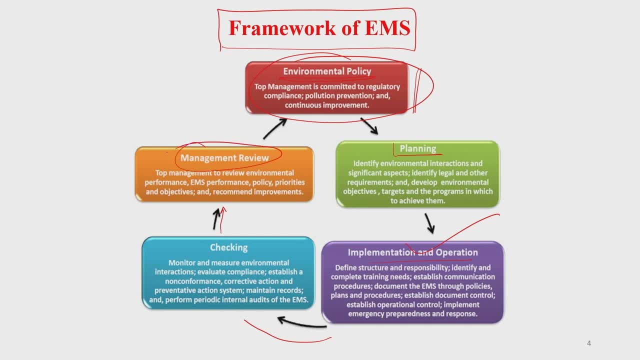 to the final, you know, review stage where top management will review the entire environmental performance. So before reaching that, during this process checking you can have minor corrections. So in management review certainly it is, kind of you know, a kind of overall monitoring or 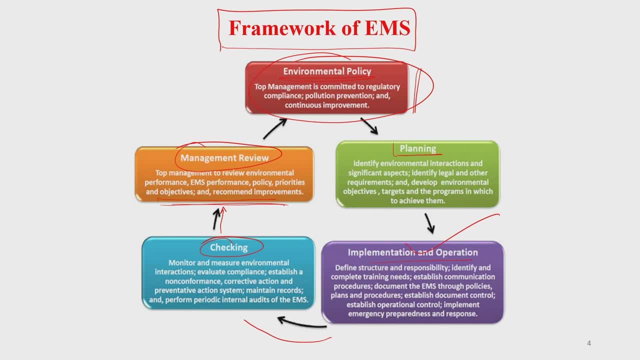 evaluation of the status of implementation of an EMS in a management. So this is the first step. Then you have to go for a certain kind of a intervention in order to actually get the ~~, the approval of the management and the evaluation of that. 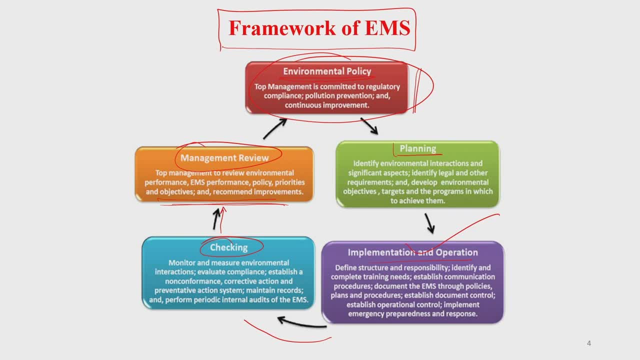 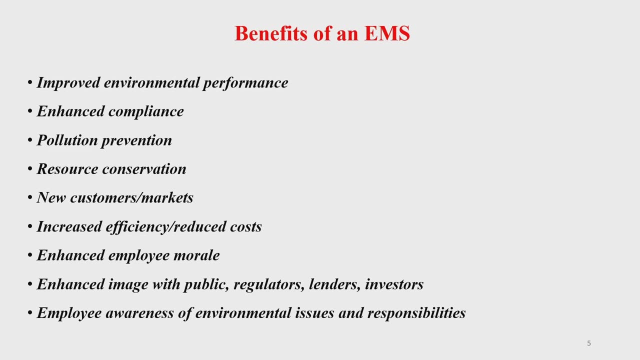 Once the evaluation has been made, then your goal is to bring the environment in the nature of the program or the environment. So you will need a lot of 2003's standards for that. and then you have to deal with the entire goal carefully and see how much others can get involved. 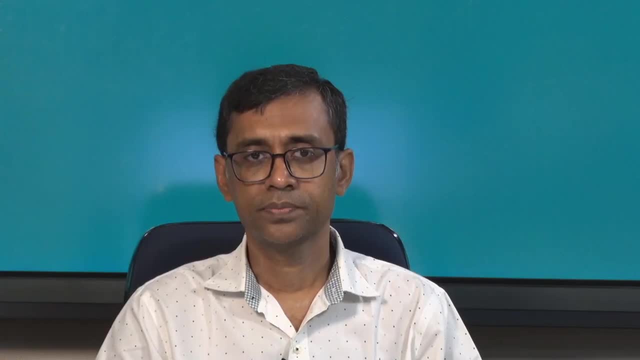 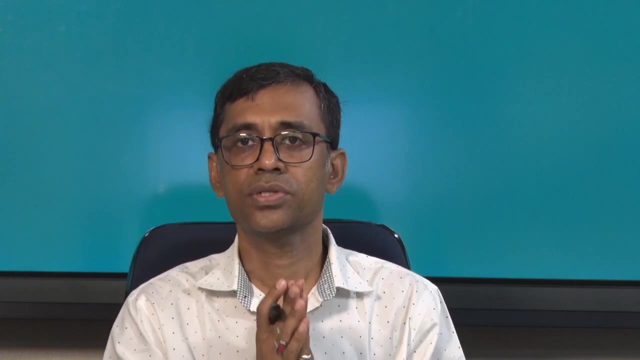 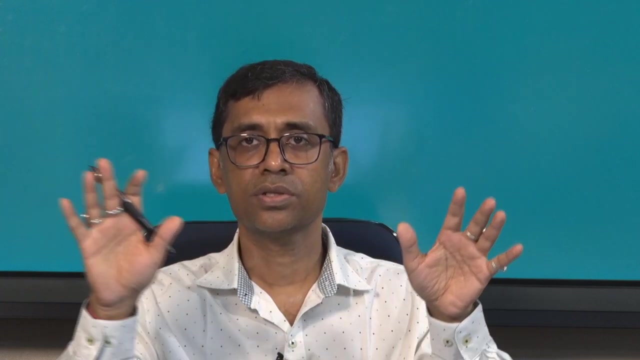 If these categories are not considered, then it will be difficult When you start being involved in the process of management, environment management system though they are. the word natural resources is not mentioned, but remember that when we talk about ems, it has a direct link or implications on natural. 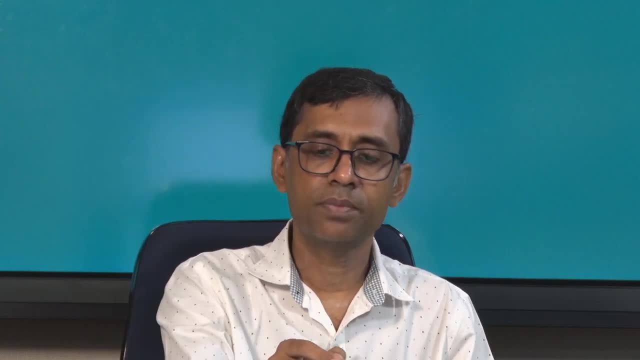 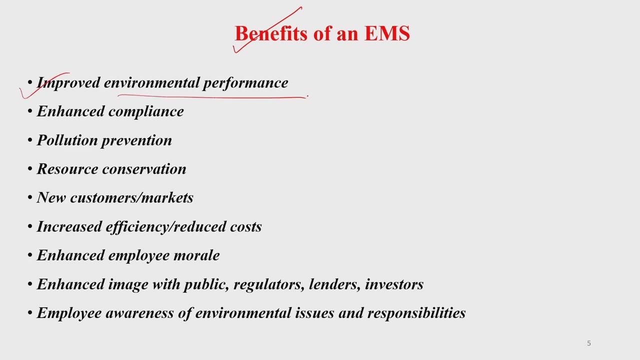 resource management as well. so let us see that. what are the benefits of an environmental management system? it helps improving the environmental performance, overall performance, of any kind of ecosystem that we talk about. it enhances the compliance of the system towards a standard. here we talk about iso 14001, pollution prevention, then resource conservation- new, you know, customers. 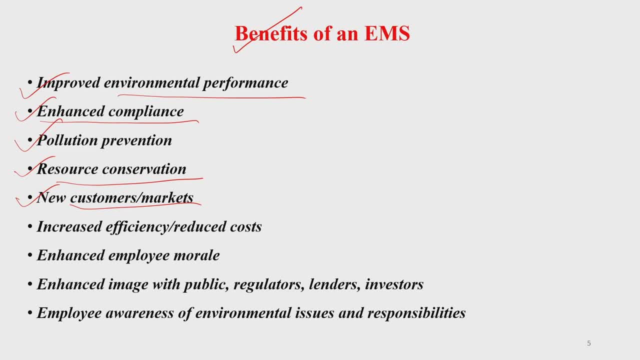 and market analysis because that will give you the extra future demand that might come in a particular ecosystem: increased efficiency and reducing cost. of course, if you increase efficiency, you, you, you know cost of managing the system expected to be going down enhanced employee model. so that is something you know you cannot create in a day or month or so, but it is a responsibility. 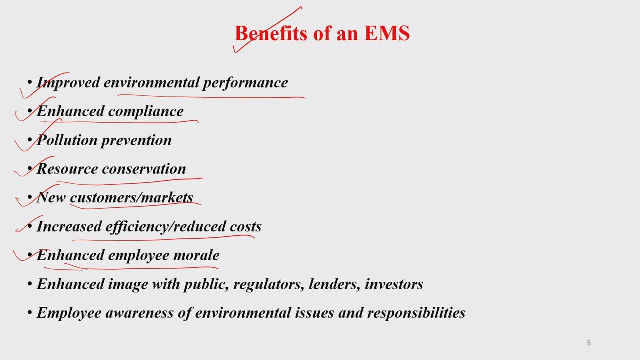 of the ems system to look at. also, enhanced model of the employee who are working within that particular ecosystem. enhanced image with public regulators, investors- because these are the people who are the key players in that ecosystem where you are working, all right. then comes employee awareness about environmental issues and responsibilities. 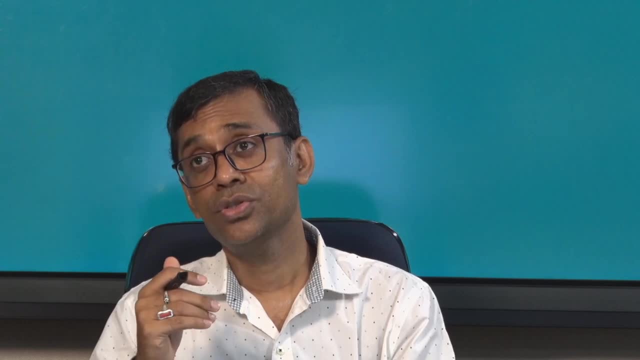 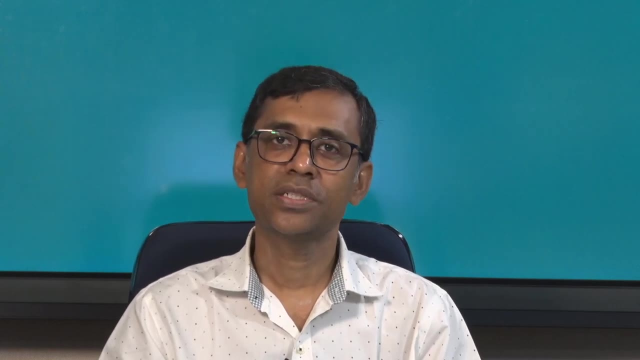 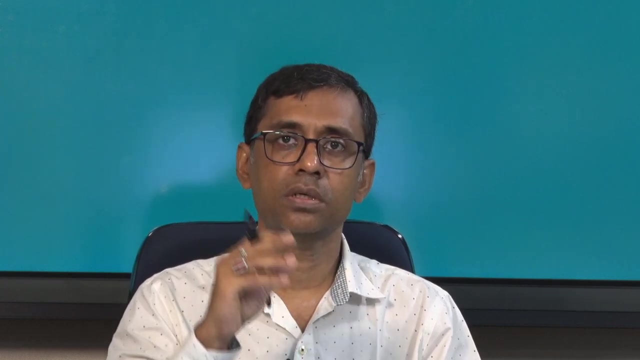 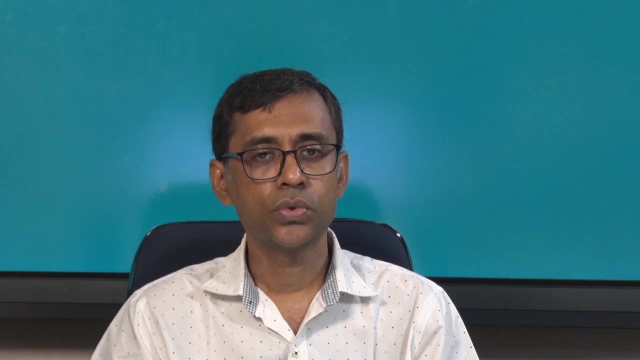 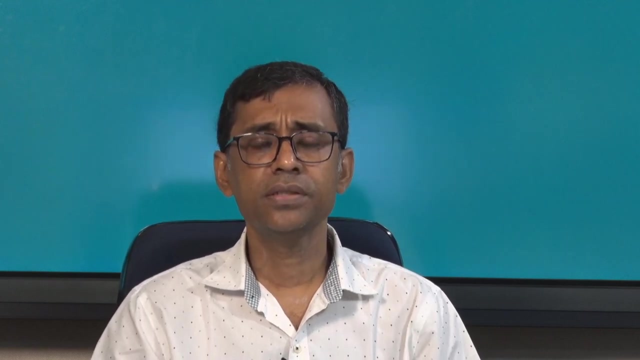 often you will find that in some of the organizations who are actually responsible for environmental management, they themselves are not aware about certain issues and aspect about environment. so it is critically important that the individuals in individuals working in this kind of systems are well aware of the issues and they should also be made about their responsibility. now. significance of environment. 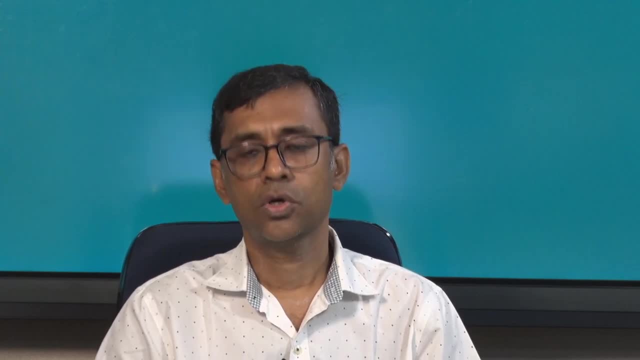 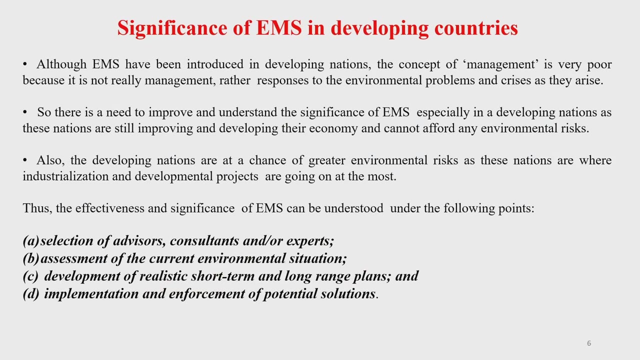 management system. in countries like India or any other developing countries. it is bit different, you know, in developing countries and developed countries for various reasons. So let us see that how EMS is important in developing countries like India. EMS have been introduced in developing nations but the concept of management is very poor because 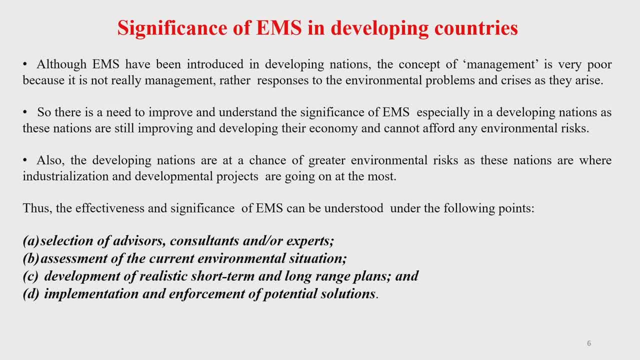 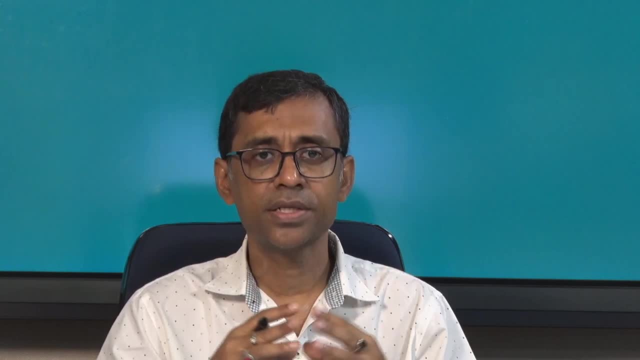 it is not really management, rather it is kind of a responses to the environmental problem and somehow you know it takes care of the problem. when it comes, arises, then it is being addressed. So in developing country EMS environment management system is little bit you know kind. 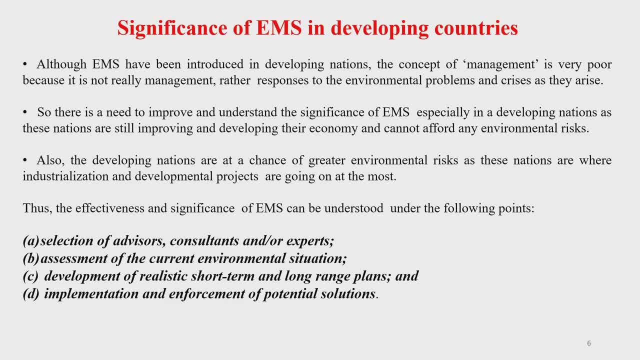 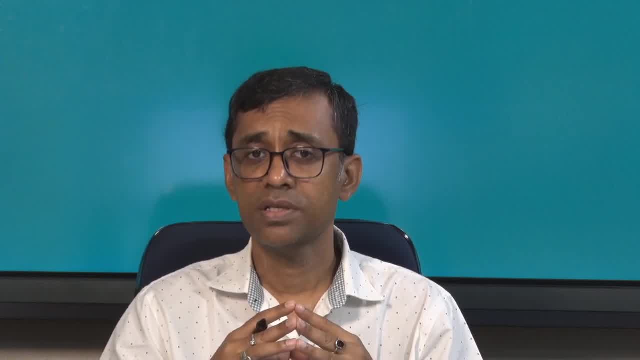 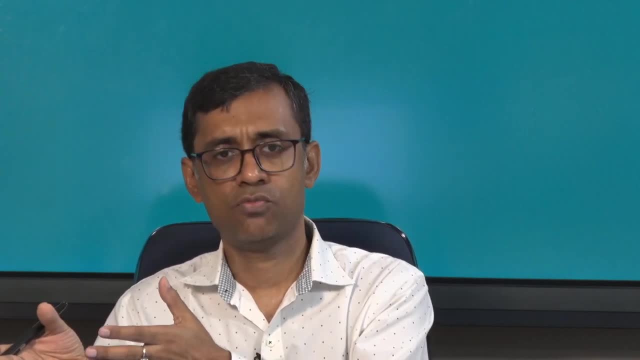 of responsive kind of or reactive kind of work is being carried out. So the principle of management at times is missing there. So that is one aspect that we need to, you know, enhance more in EMS framework: the management aspect. So there is a need. 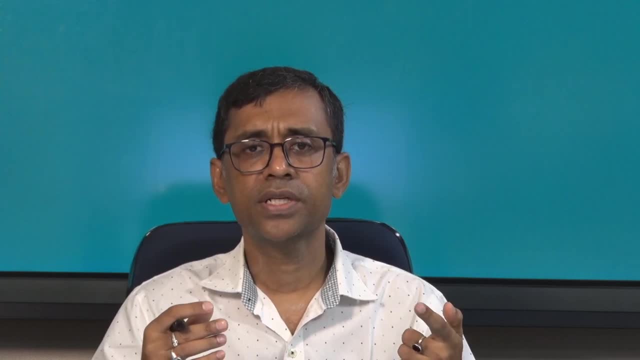 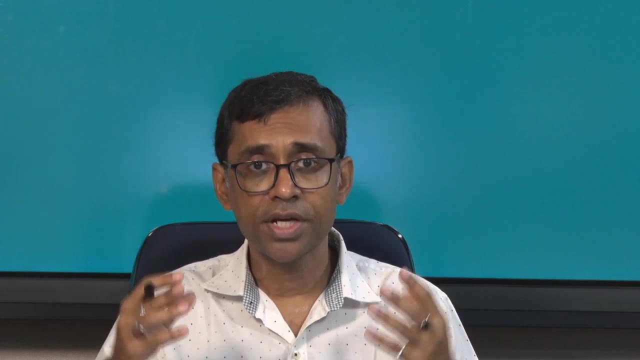 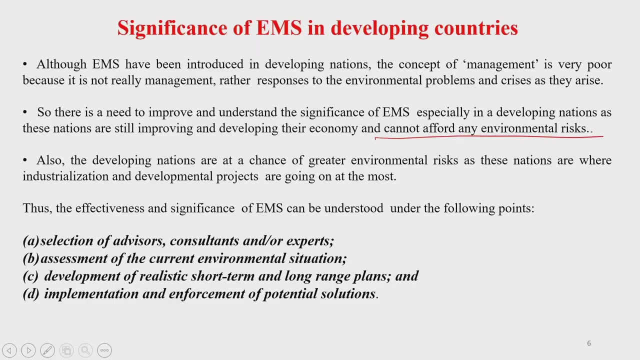 to improve and understand the importance and significance of environment management system, especially countries like us where the economy is still growing, and growing at a very high pace. So we cannot afford any kind of- you know- environmental risk because that would be very- you know- disastrous for. 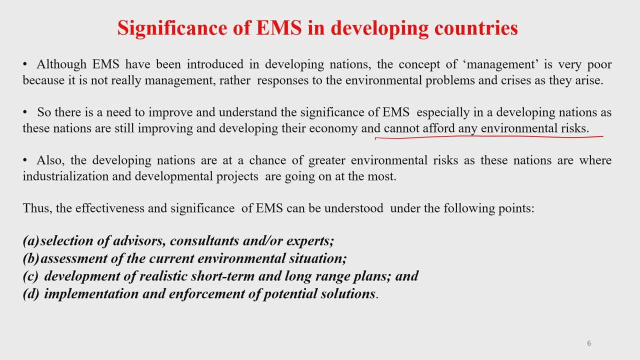 our, not only our- environment, but also the development growth path that we are following. So, for the betterment of our own growth, it is important that we try to apply the environment management system in appropriate manner, So the management part which is little weak or poorer still, 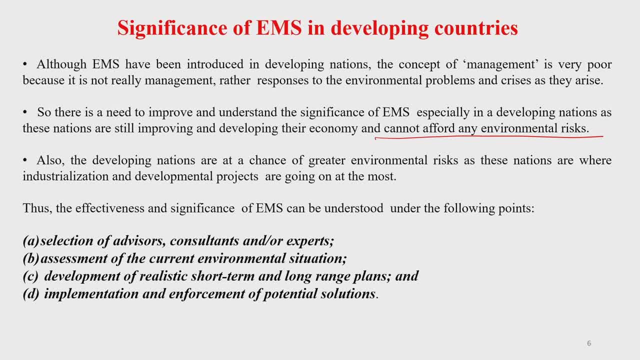 in many parts of our country that needs to be taken care of. Also, you will find that the developing countries are at a chance of, you know, greater environmental risk for various reasons, probably for our geographical locations, etcetera. I am talking about almost all a. 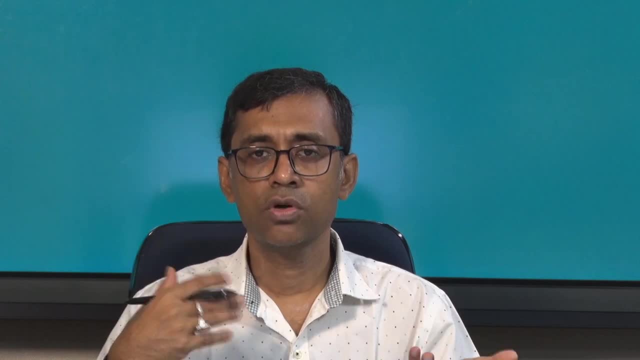 developing countries. So they are also having some natural- you know- expose to natural risk, and these nations are where the industrialization and developmental projects are going on at the most. So you see that such a hub, I suppose In overall you do not have to think of industry. 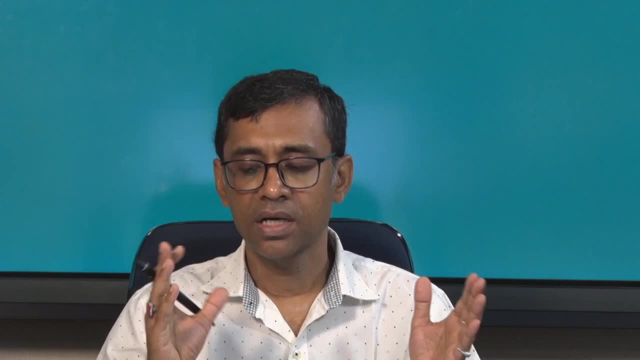 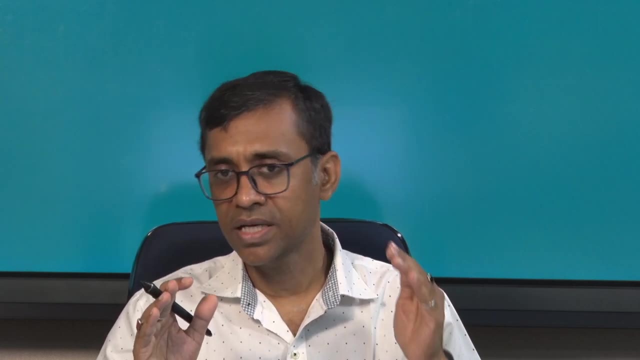 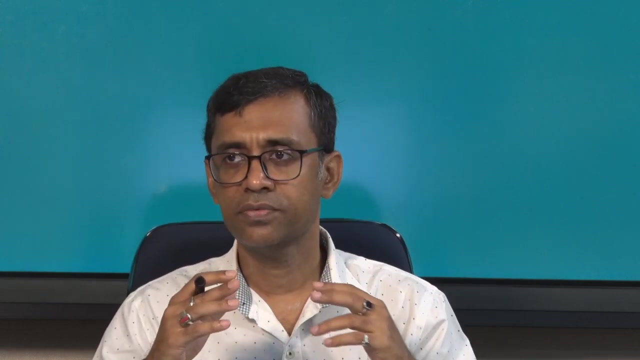 it is bringing the terrific idea of it to the national system. So can you comment directly that the countries are already having certain inherent environmental risk? but these developing countries are actually at the you know path of very speedy development, growth. Industrialization is taking place, various kind of infrastructure development, So the inherent risk or entrenching, 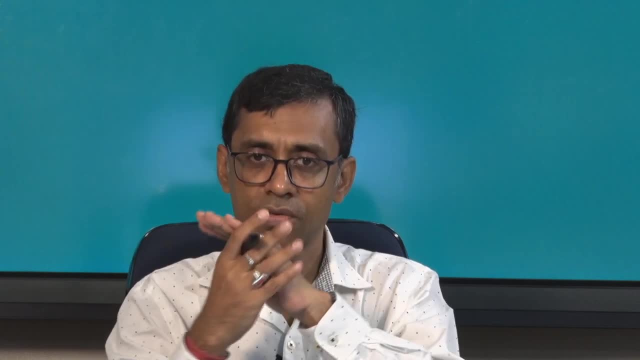 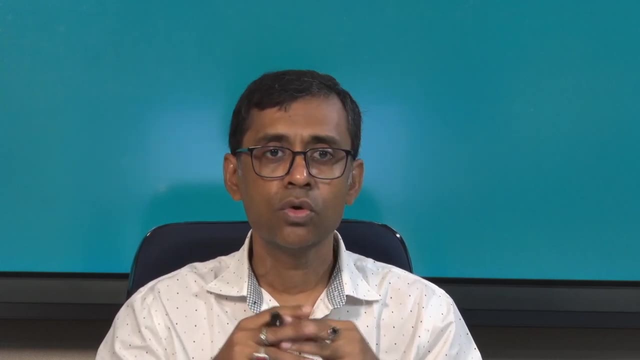 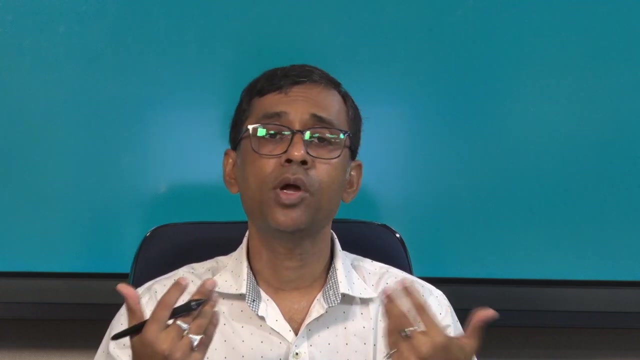 risk plus this rate of growth, So there of course there is a chance of more risk in those kind of areas. So we must have a very robust EMS system so that our own design, development, growth is not hampered because of this kind of risk, which are already there. 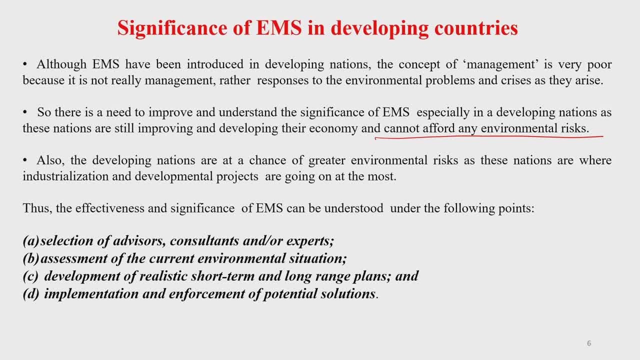 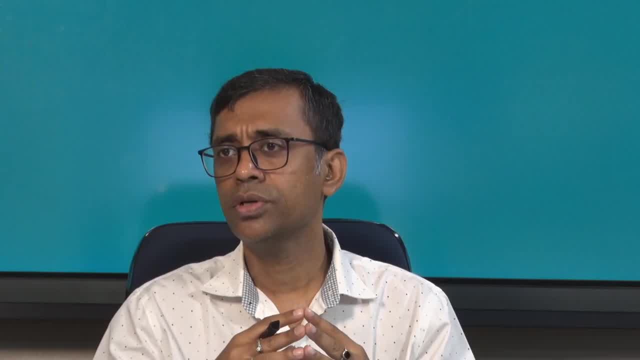 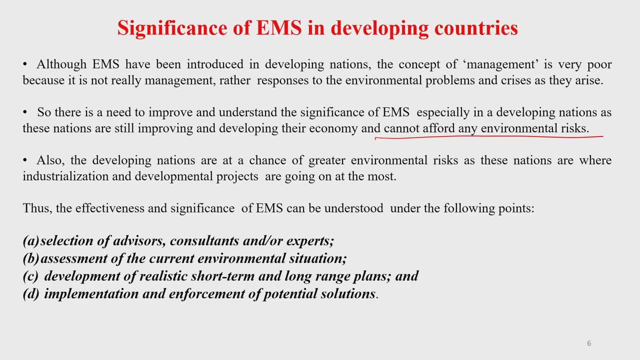 in the system, plus because of this first you know- plan of growth. Then the thing is that we are actually at the- you know threshold that we need to take care of our EMS in a very effective manner, As I again, I repeat, the management part of 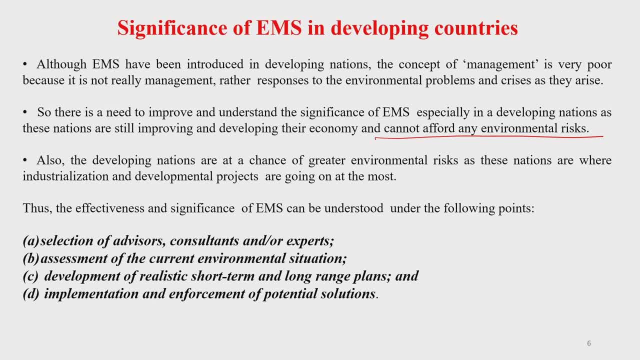 EMS need to be strengthened and EMS significance of EMS in our society. it actually need to be understood very clearly and to do that we need to do, you know, some kind of initiative And some kind of activities planned in our society and ecosystem. Selection of advisors. 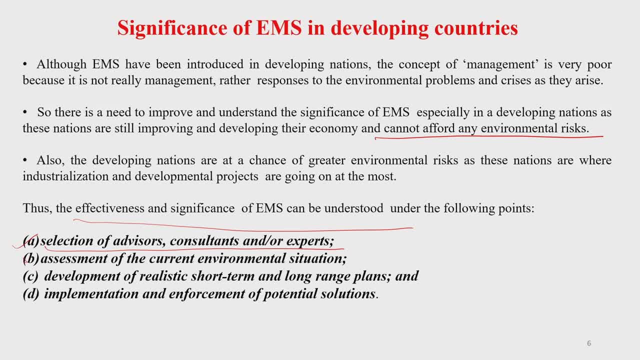 consultants and experts is one way to do that. assessment of the current environmental situation. This also will tell you the effectiveness and significance of EMS development of realistic short term and long term plan. So you have two sets of plan in hand, Plan which actually 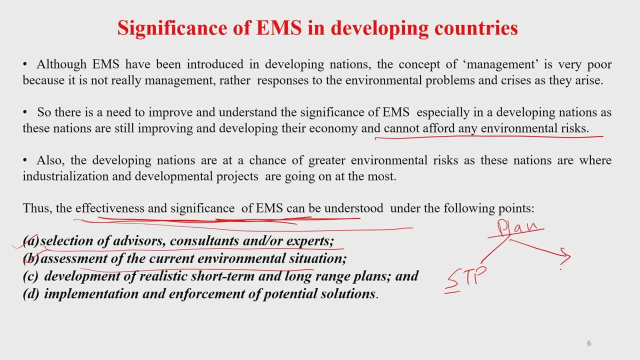 you know you might like to bring those two to memory because you know, if you want to know, you can easily address within a very short period of time short term plan and another is long term goal. So these two things need to be taken care of, and then implementation. 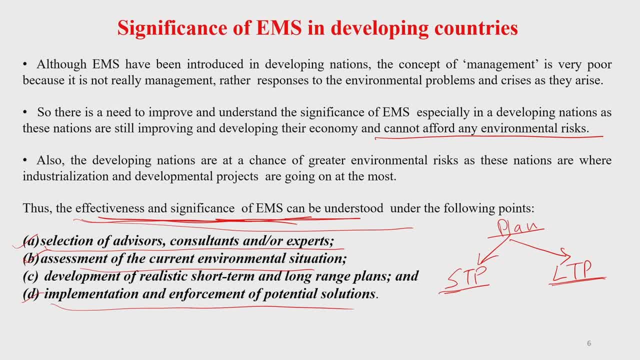 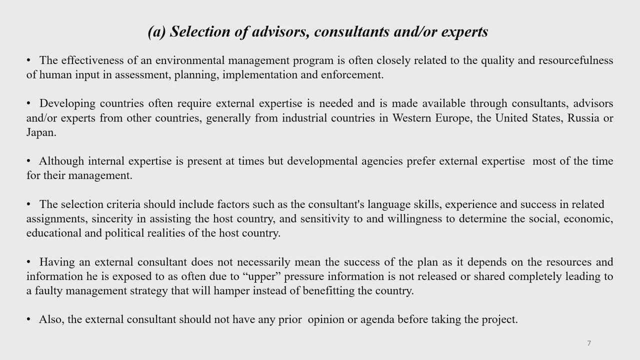 and enforcement of potential. you know solutions. So, even if you identify certain potential solution, the important matter is that how do you implement that and also enforce that solution into the system that you are working with Now? this selection of advisors and consultants and experts is a critical step, and this has 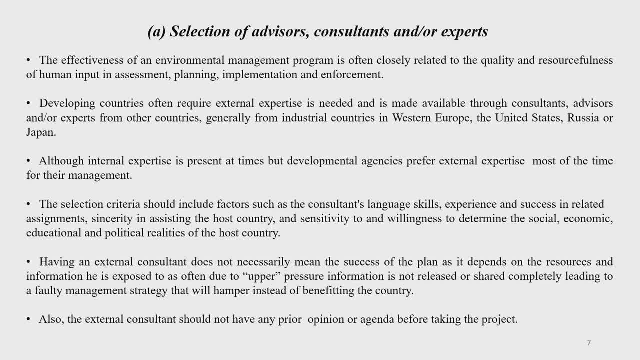 to be, you know, done with lot of care. The selection criteria, you know, should include various factors, such as the concentrated language skill, his expertise, Experience, knowledge, sincerity, etc. etc. and his knowledge about the particular area. 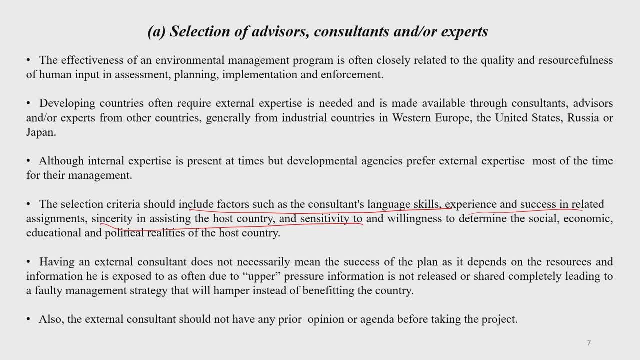 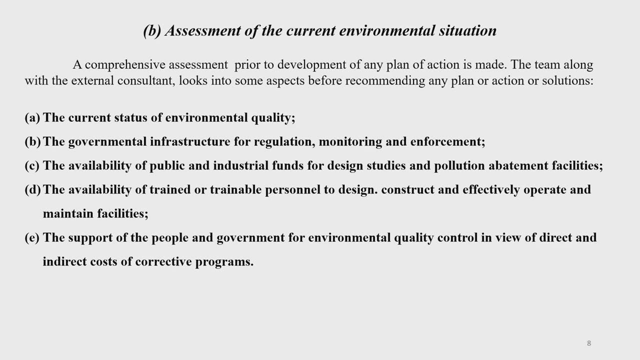 the location and also the person, expert or advisor should not be having any kind of bias or kind of, you know, prior opinion and agenda before getting into this kind of project or work. Then next, this assessment of the current environmental situation is also you know, 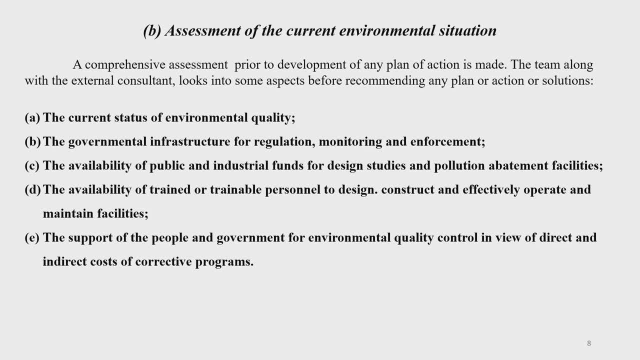 can tell you the efficiency or effectiveness of your EMS system. So a comprehensive assessment prior to the development of any plan need to be made and the team, along with the external advisor or consultant, they should look some aspect before recommending any plan or action for the solution. all right, 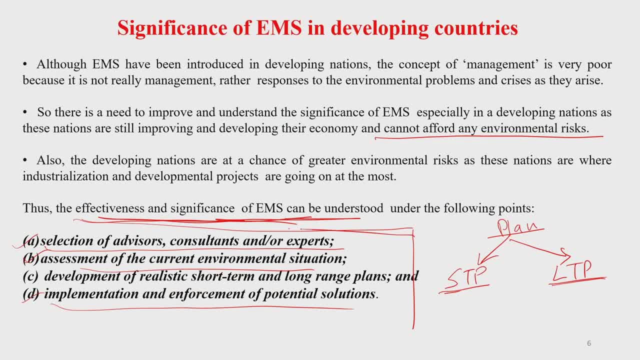 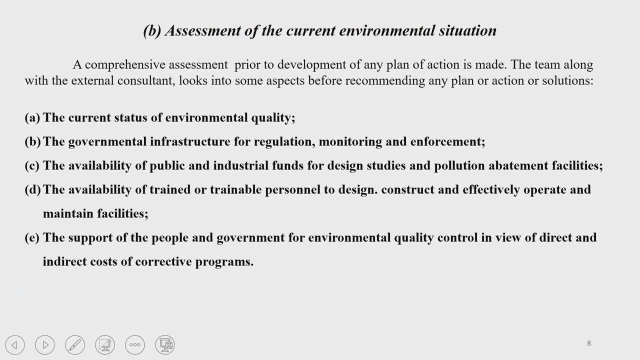 So I go back. So here I was talking about that. this is the some way that you can actually understand the effectiveness and significance of EMS, and here we are talking one by one, That how actually you can carry out these exercises. So assessment of current environment. 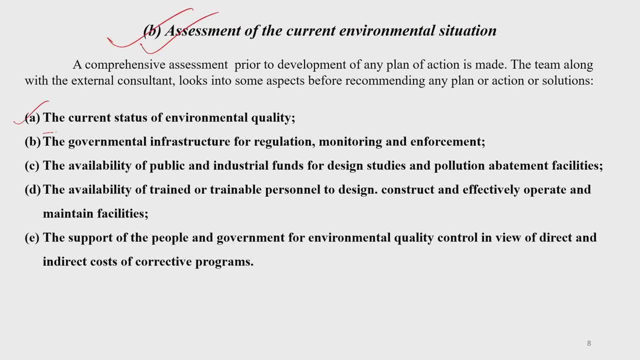 situation is very, very important. What actually you have to do? We have to do the study of current status of our environment quality. That will be our baseline. Then we should look at the- you know- governmental infrastructure for various regulation monitoring. 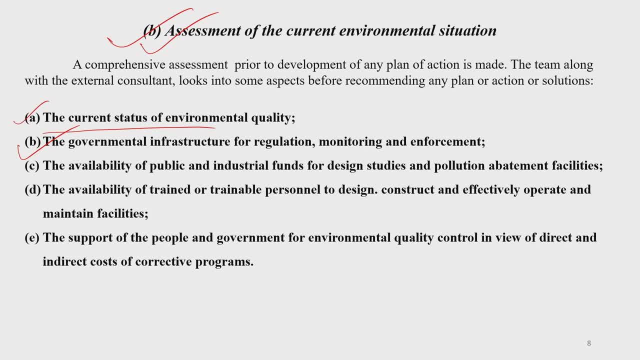 enforcement, because within that government set of many things will be taking place, So need to also understand that very carefully. Availability of public and industrial funds that need to be utilized for various activity, because that idea will give you that how you design your course of actions and also different other activities associated with environmental. 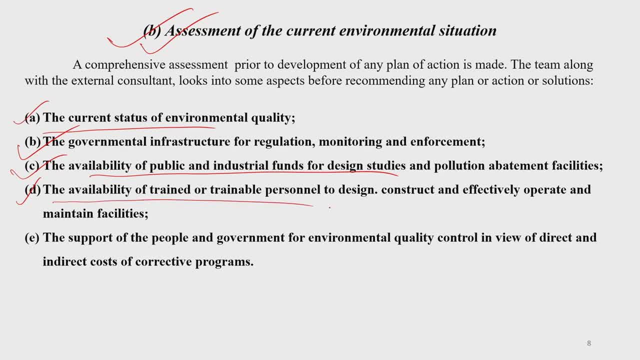 management. Next, the availability of trained or trainable personnel to plan, design, construct and effectively- you know- carry out this action. This is where, often, we find, at the field level, you will find the challenge At the proper time to find a skilled person for a particular work. 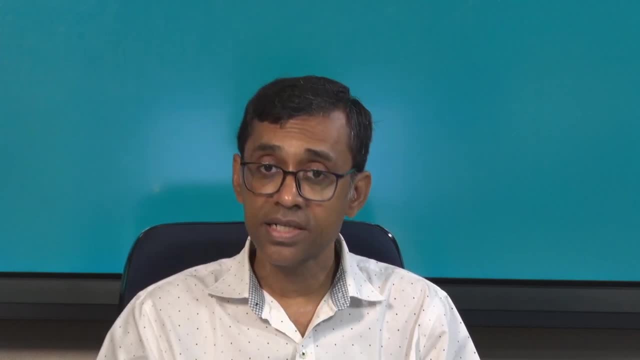 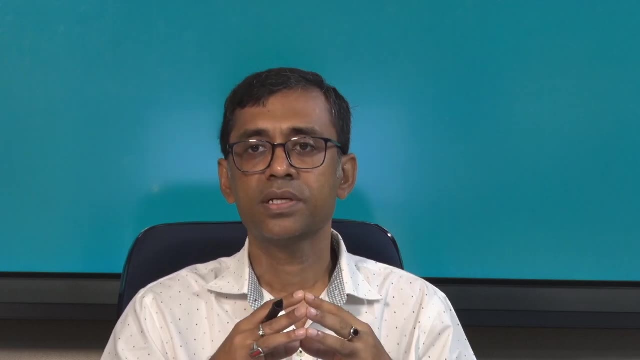 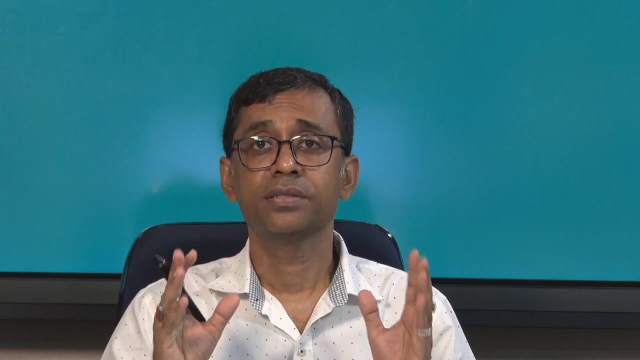 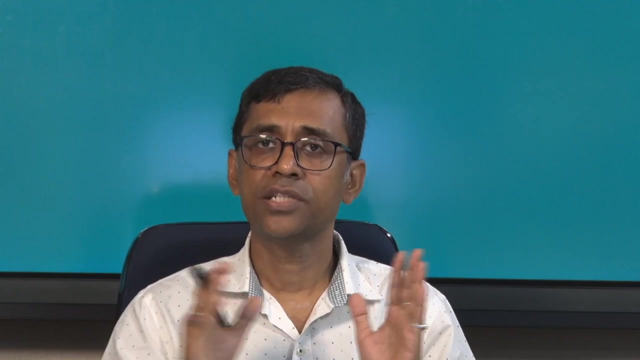 you will see, you will not find that, and that is why many times this kind of work related with natural resource management, environment management system get badly affected. So we need to have a pool of trained, skilled personnel for that. the preparation should start long back and 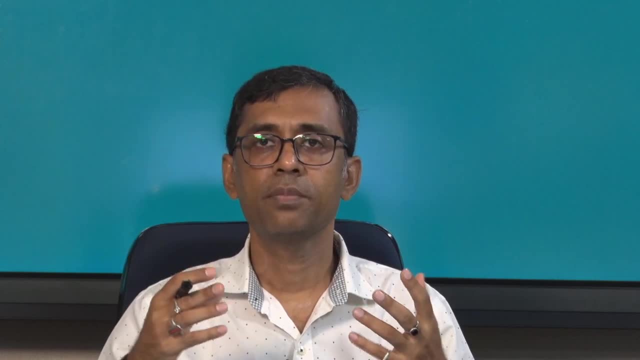 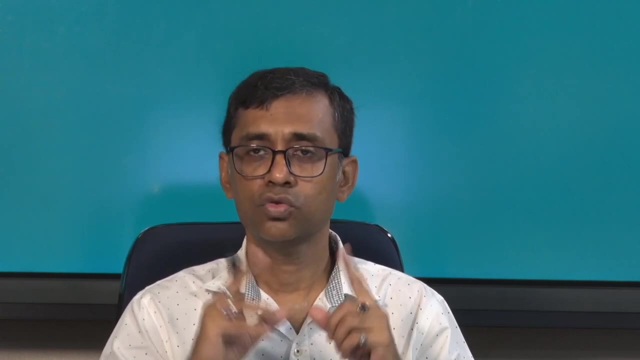 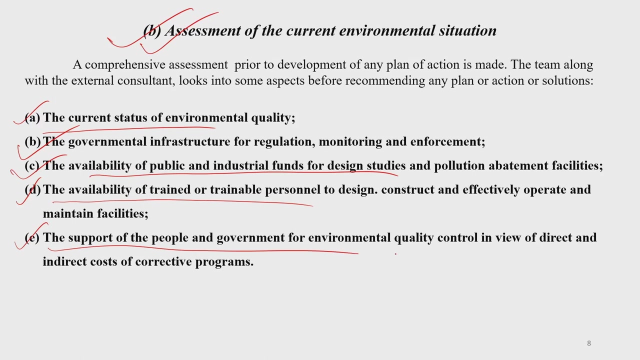 it should be a continuous process. Process of skill development for natural resource management, environment management system should be a continuous process So that, when the need arises, you have a set of people who can actually carry out the work. The support of the society, the people, the government, the 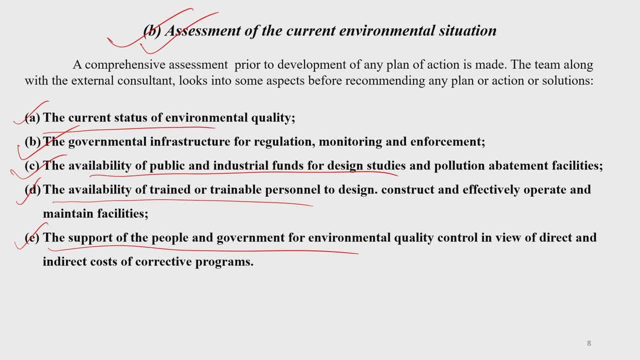 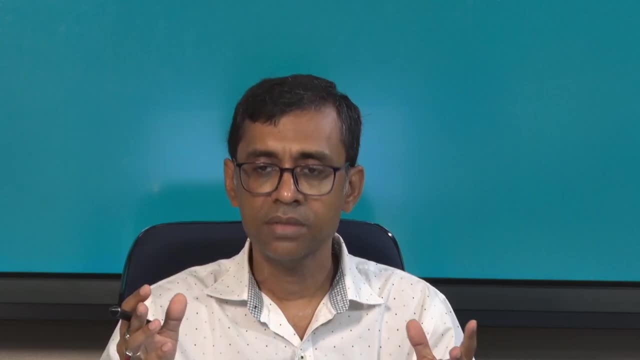 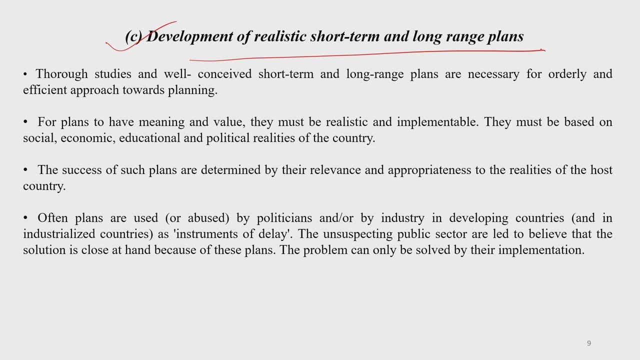 environment is very, very important for maintaining environment quality, to manage the natural resources of any ecosystem, because without the people support we cannot carry out a very effective or efficient environment management system, and so the natural resource management system. Next, development of realistic short term and long term plans- very important, as I said. 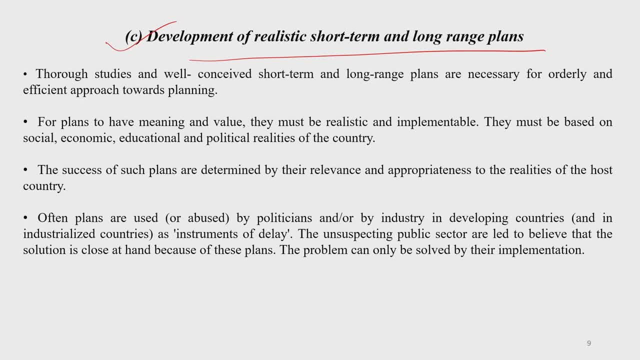 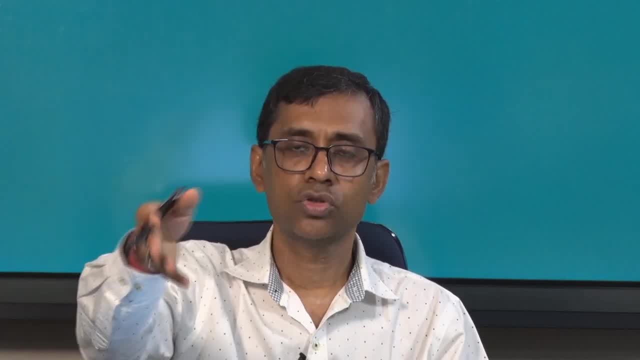 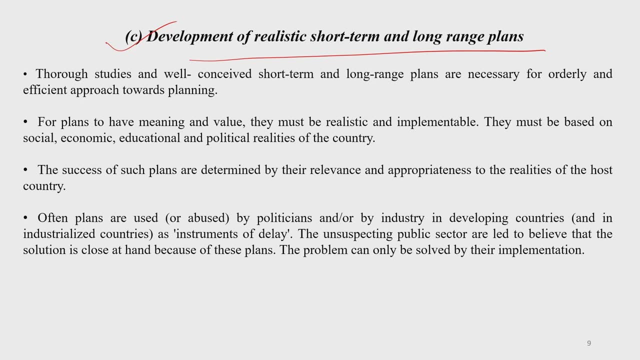 that have in one hand, short term plan, which we can finish, suppose, within few months, a year or so, and then we have a long term plan, couple of years. So these two set of plan should be envisaged, prepared through consolidated studies. So once you know these kind of plans, 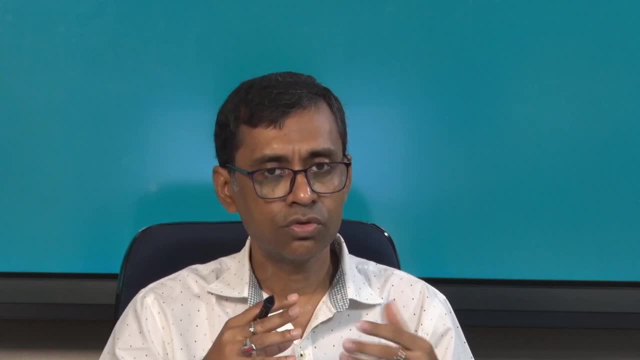 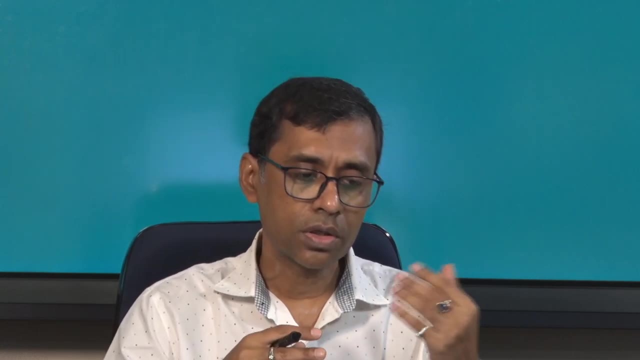 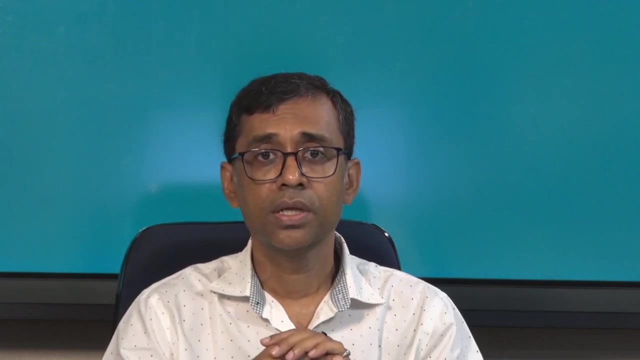 are kind of ready and it is ready in your hand, then to carry out a very efficient EMS or NRM will be very, very easy. So for plans to have a value for the society, for that particular ecosystem while you are working, they must be based on realistic and implementable ideas. So we must know the 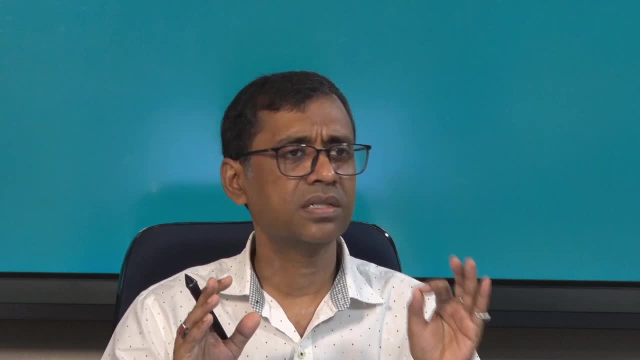 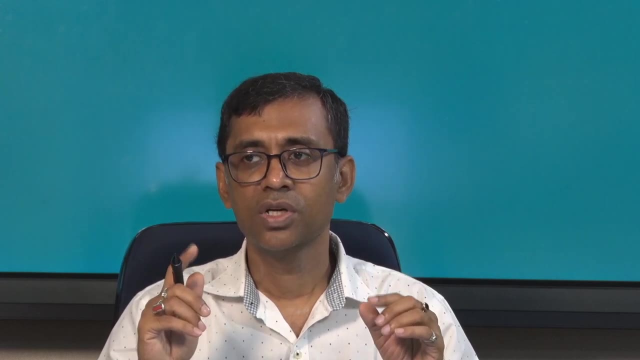 place and the area and then think about certain realistic target, real and implementable ideas. there must not be, you know. they must not be based on some other assumption and that is why you know. 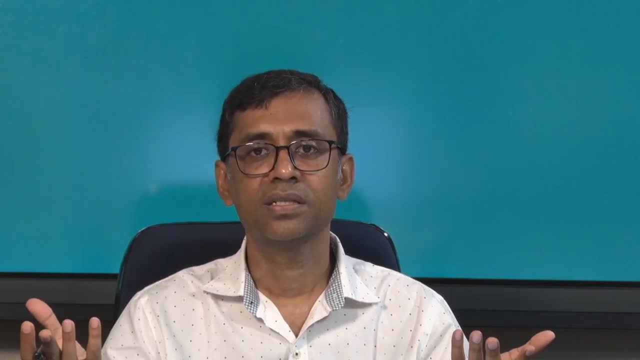 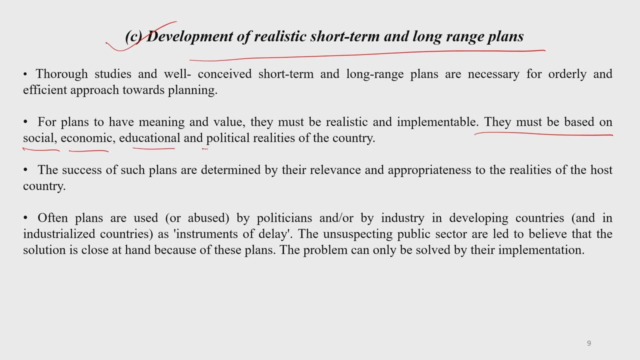 consolidated study and knowledge about an area is very important. So these plans, they must be based on social, economic, educational and political realities of the country, of the area where you are working, And the success of such plans will be determined by their relevance and appropriateness to the real condition of the ground. So if your conceived 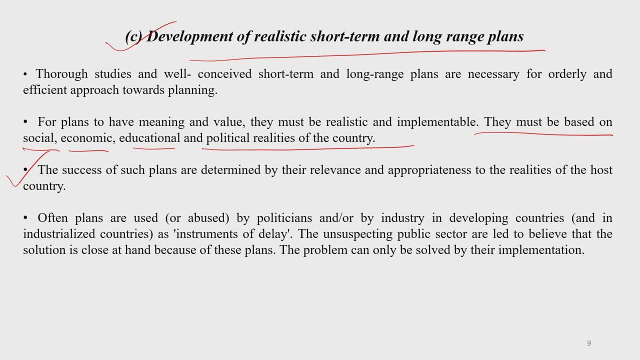 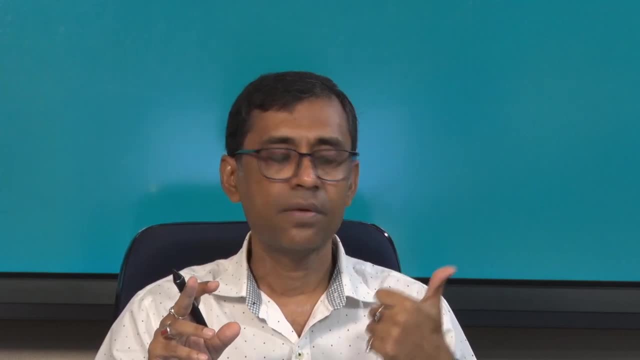 idea or plan is made, sitting far away from the area where actually the plan will be implemented, I am sorry. there is a high chance that the plan will fail. So we must be very realistic and our plan, whether short term or long term, it must be. 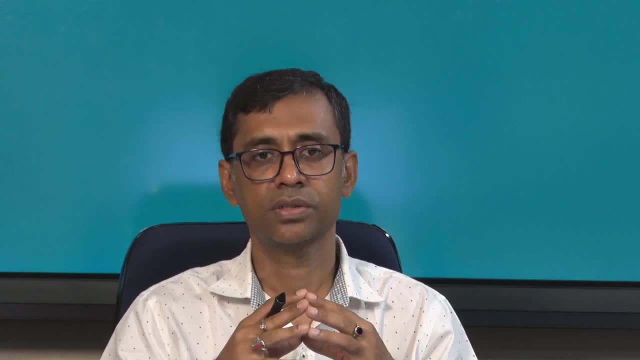 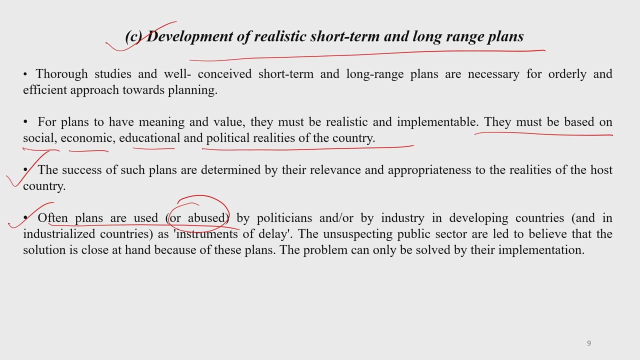 based on the real grounds situation. Often plans are used or abused, you can say, And sometimes it is used by politicians, stakeholders, different people from industry in developing countries and sometime also in developed countries. So what happen is that sometime these initiatives 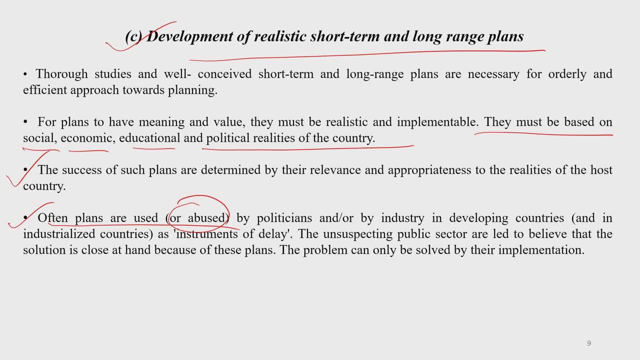 activities get delayed for some unknown reason. Now, the unsuspecting public sector are often led to believe that the solution is close at hand because of these plans. But the problem is the problem is not the public sector, the problem is the public sector itself. So 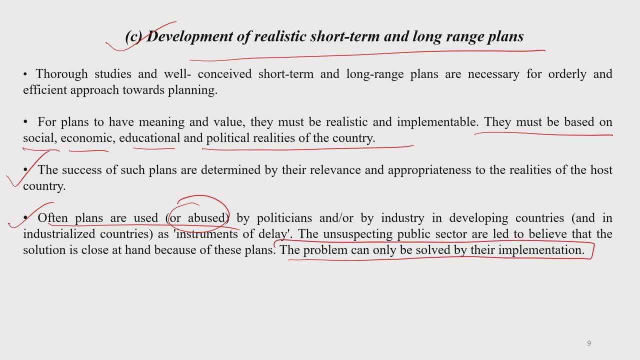 problem can only be solved by their implementation, not by the planning, not by hiring consultations only, but the problem can only be solved by their proper implementation on the ground. And this fact is true for any country across the world, developing or developed world. 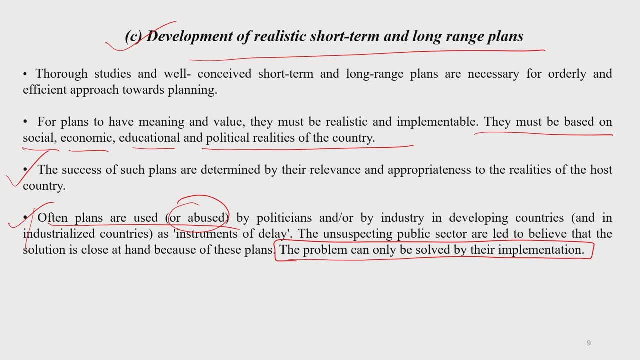 So this is also one aspect, because we are working with all natural resource management specialists. we will be working in this society only. So we must be aware of this real fact and accordingly devise the course of actions so that your process, implementation process- 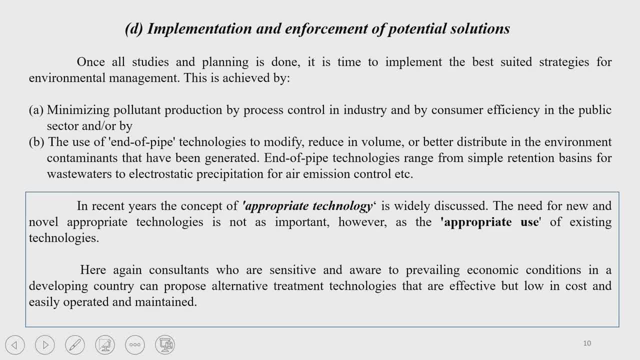 or actions is not delayed due to some other external factors. Next, implementation and enforcement of potential solution. Exactly this is what I just discussed in the previous point. Once your planning is done, it is the time for implementing it, And this is the most critical step. So you will find that in recent years, the concept 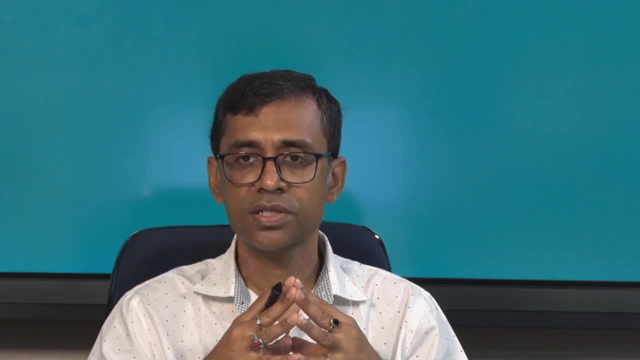 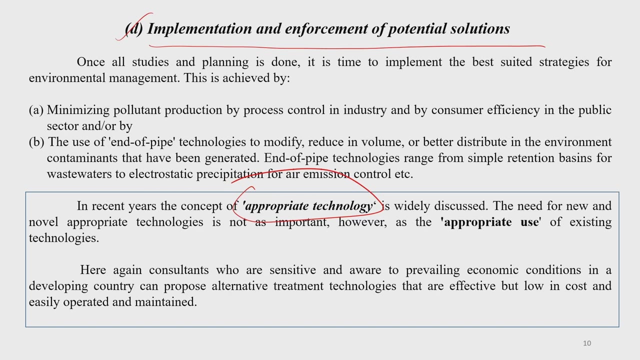 of appropriate technology is often discussed in various forums- appropriate technology. So the need for new and novel appropriate technology is not as important. However, the appropriate use of existing technology could be very, very important. I repeat it: the need for new, 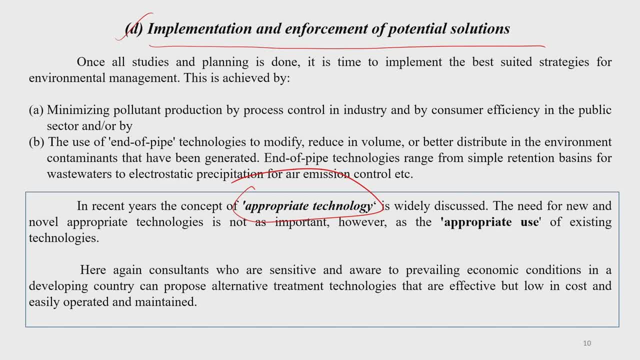 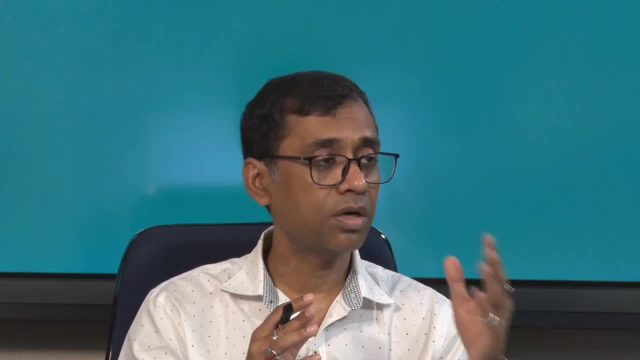 And novel appropriate technology may not be as important when you compare with the appropriate use of the existing technology. So we have certain amount of technology- any society you know, even including the indigenous technologies- with the community. So it is important to 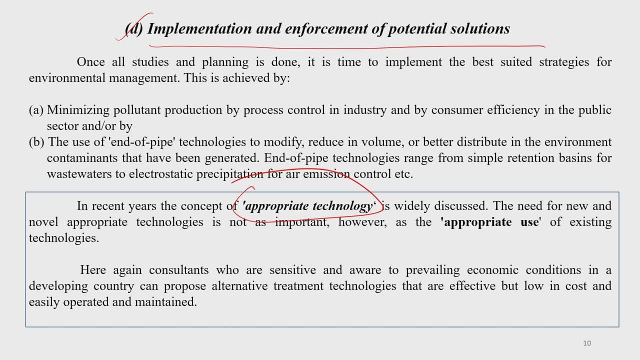 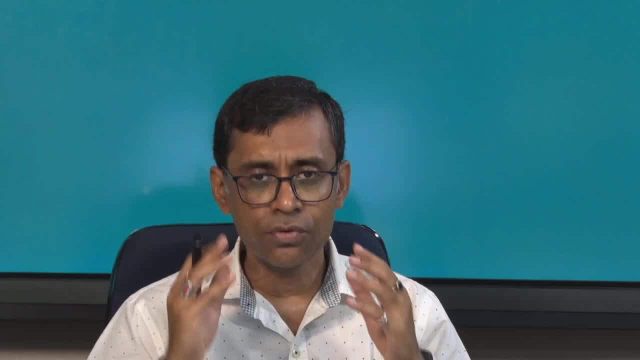 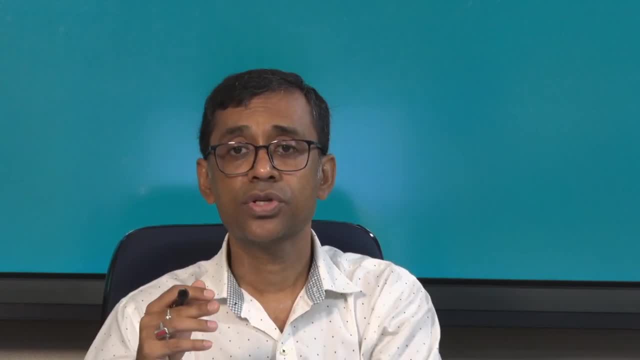 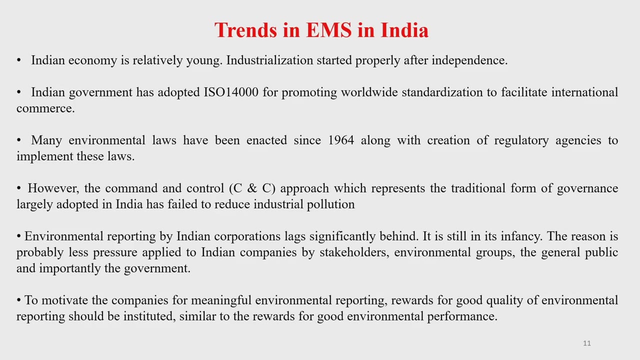 see that the appropriate use of those technologies which are already in the shelf with us is being carried out. Of course, appropriate technology off the shelf is equally important, and for that research and innovation need to be carried out. So next is trends in EMS in India. So if you look at that, environment monitoring systems. 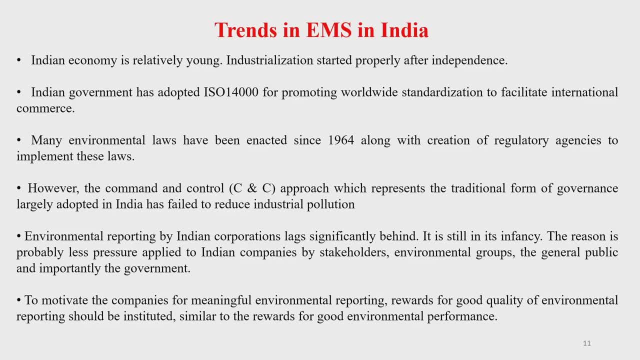 and its trends in our country, you will find that Indian economy is relatively young and our industrialization has started in a proper manner. That is why the goal of EMS is you should have a standardized economy, which is very important Every time in India. India is still a kind of a high standard, So the buildup of the 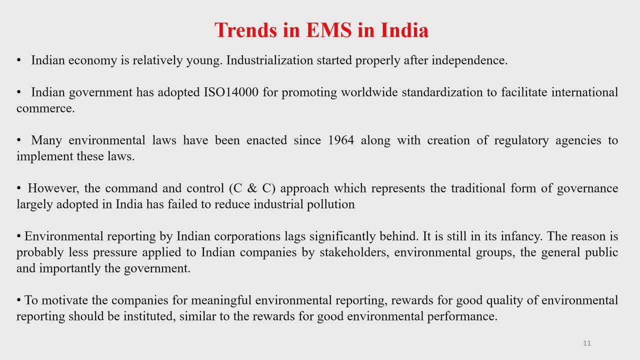 industrialization is always very, very important, as you have seen in our analysis, and that is why it has been recommended to use international standards. So the urbanization is very, very important. The urbanization is very important. So the urbanization is very, very important. There is hardly any kind of a standard in India. The urbanization can be it for the reasons they can be all about. On the other hand, if you know, if you have a country like India and you know that the market is very, very big and the environment is very, very big, then you need an economy to maintain. 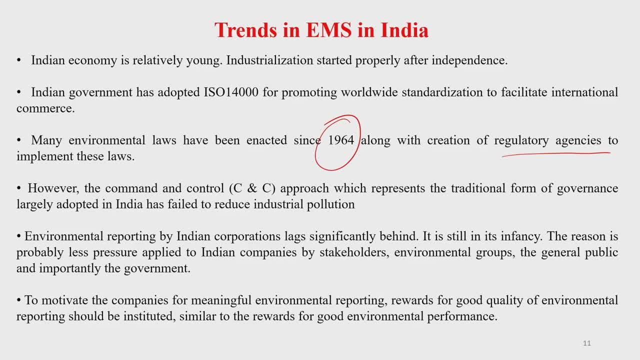 the modernization of the country made this kind of law. However, the command and control, which we call CNC. this command and control approach, which represents the traditional form of governance that has been adopted in our country, has somehow not been successful in reducing the industrial pollution. 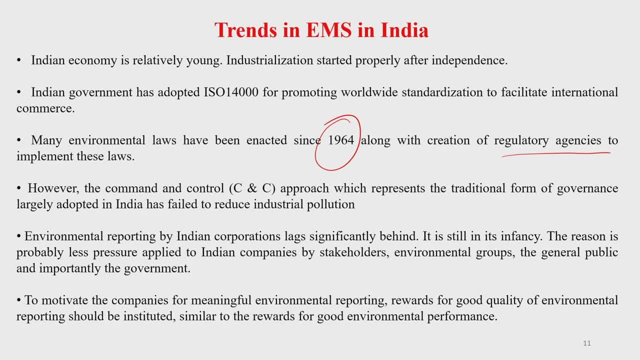 Now there are various reasons for that. Perhaps most of you might be knowing if you are following. you know print and you know television and other kind of media. Environmental reporting by Indian corporations also lag significantly behind. you know the corporations in developed countries. It is still in infancy. There are various reasons for this. Probably you know less. 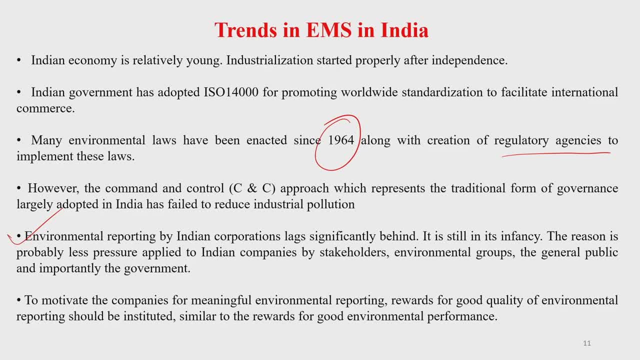 pressure applied by our Indian companies, by the stakeholders. So our stakeholders need to become more proactive and these companies should be more proactive, Should be answerable to some of the queries generated by stakeholders, environmental groups, general public and, importantly, government. So this kind of system need to be in place. 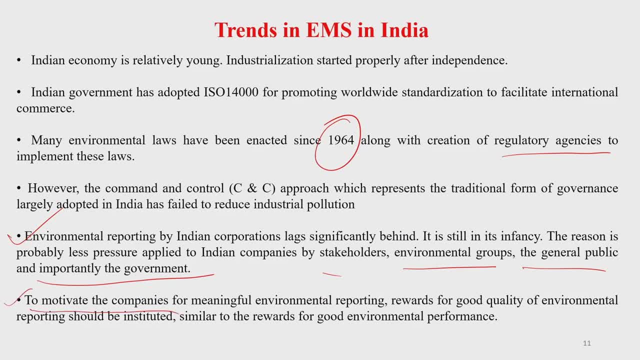 Then EMS is also important to motivate the companies for meaningful environmental reporting. Rewards for good quality of environmental reporting should be instituted, Similar in line of, you know, rewards for good environmental performance. Now, this kind of thinking and process need to be more frequent, visible, so that every 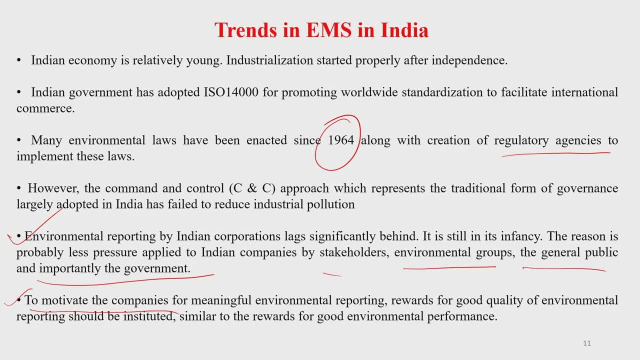 individual companies or corporates, industries, they automatically take this kind of system blended with their already existing different kind of management system within their organization. EMS should not be a kind of a standalone management system within an organization or industry or a company, So that needs to be ensured. 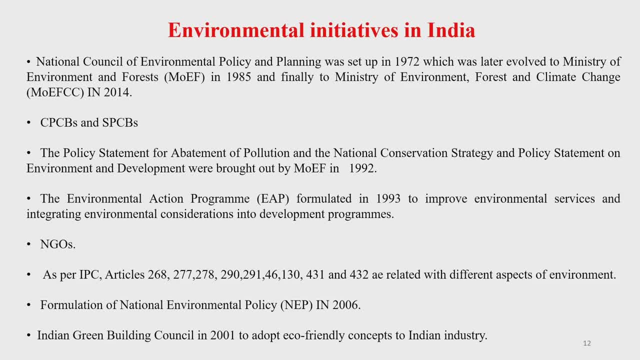 If you look at the various environmental initiatives in India: our National Council of Environmental Policy and Planning, which was set up in 1972, which was later evolved to Ministry of Environment and Forest, or MOEF, in 1985. And finally, to Ministry of Environment, Forest and 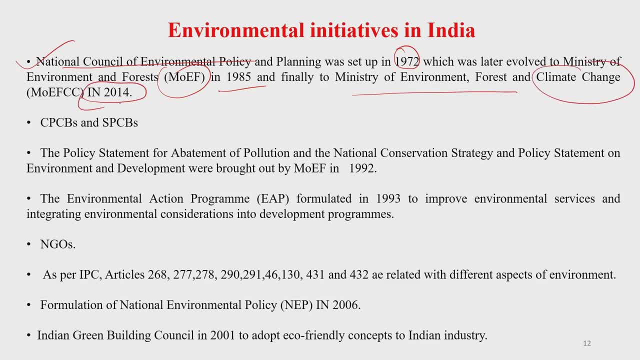 Climate change recently in 2014.. Under various There, there are assuming that new industrial developments and Various initiatives. there are also CPCBs and SPCBs has been created: center pollution control board, state pollution control board, Then the policy statement for abatement of pollution and the national conservation strategy. 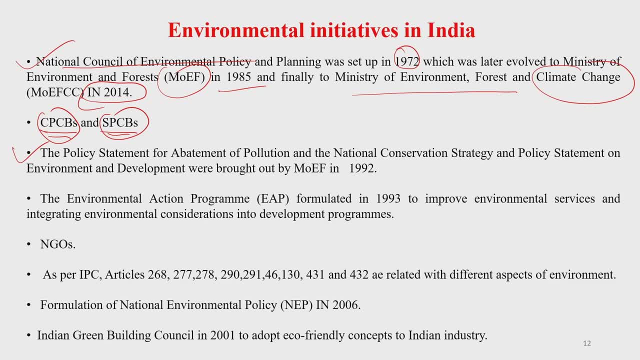 and policy statement on environment and development were also brought out by MOEF in 1992.. The environmental action program, EAP, another very important initiative formulated in 1993 to improve environmental services and integrating environmental considerations into development paradigm of programs. NGOs working in the field of environment did come up one as one of the, you know, conscious 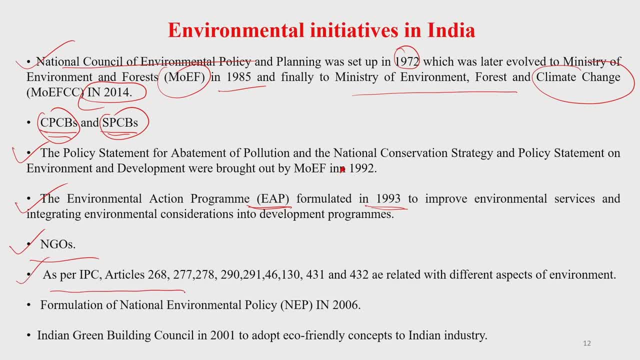 effort of the government As per IPC articles 268,, 277 and 278.. And etcetera, as mentioned here. These are all related with different aspect of environment and also been looked into and formulated. Formulation of national environmental policy, or NEP, in 2006 is another very important achievement. 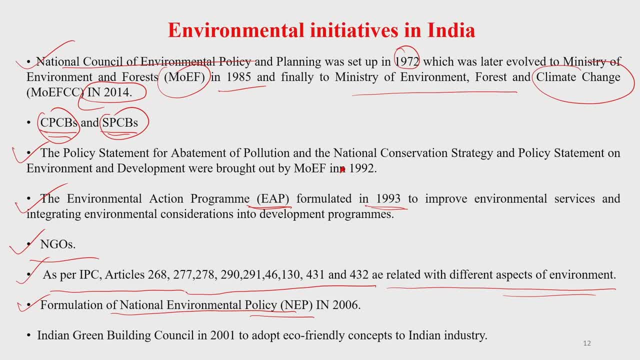 or I say milestone, under environmental initiatives in India. Indian green building council in developed in 2001 to adapt eco friendly concepts to Indian industry. This Indian Green Building Council is very, very important, especially nowadays when most of the cities, the metro cities, are coming up with, you know, huge number of buildings.